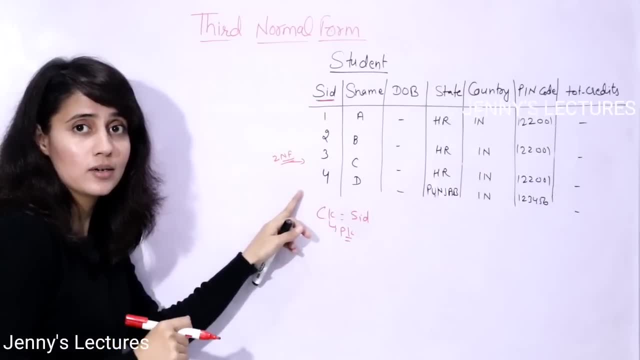 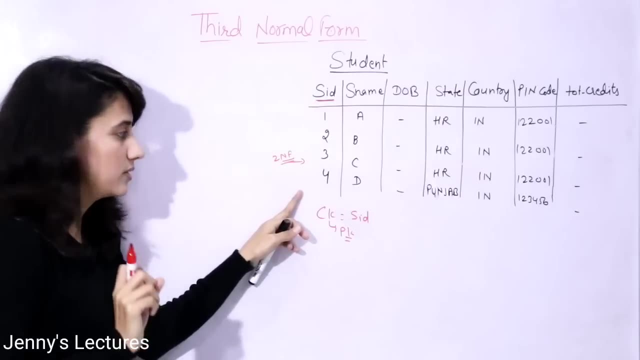 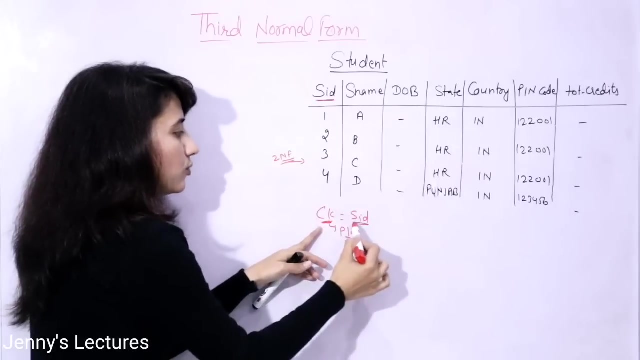 given any functional dependency right And in the previous video I have checked using that functional dependency right. In the previous video I have told you one more important point about second NF is that if the candidate key right is having only one attribute, 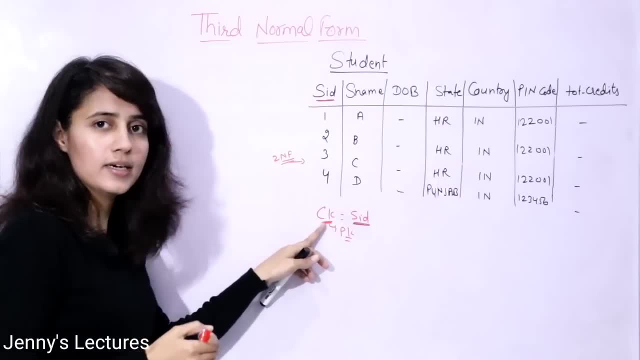 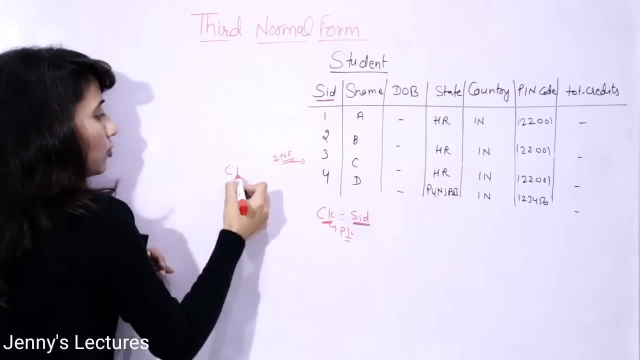 although, luckily, we have only one candidate key. suppose three candidate keys are there and all three candidate keys are having only one attribute. See, candidate key is also having one attribute. If candidate key is having one attribute, then that is. you can say simple. 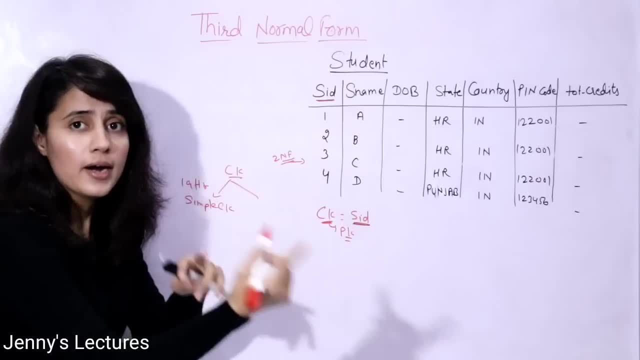 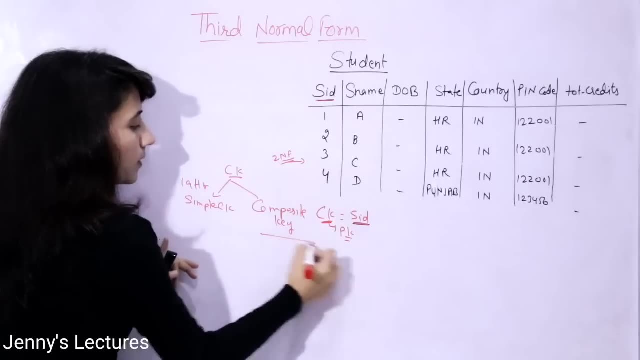 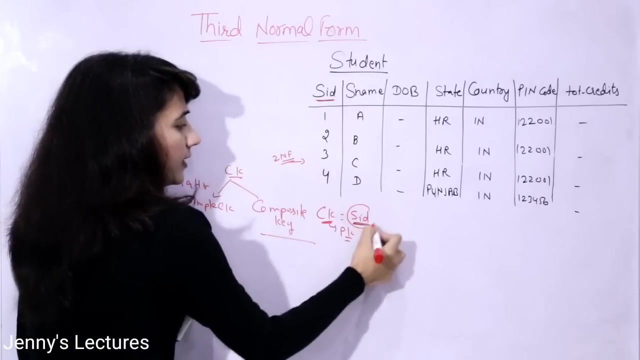 candidate key If it is having more than one attribute- two, three, four, five, six, seven, ten, eleven total- then that is known as composite key, Right? I hope you got now what is composite key? Now see, if the candidate candidate key is having only one attribute, then definitely. 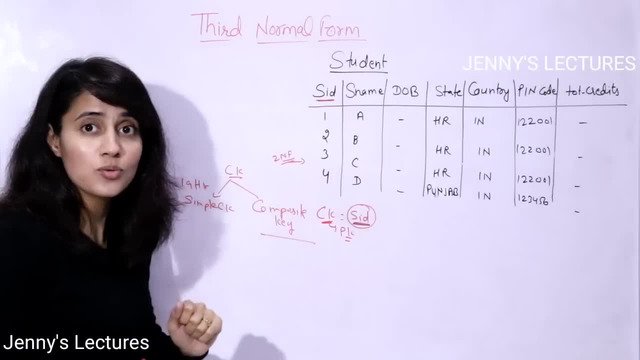 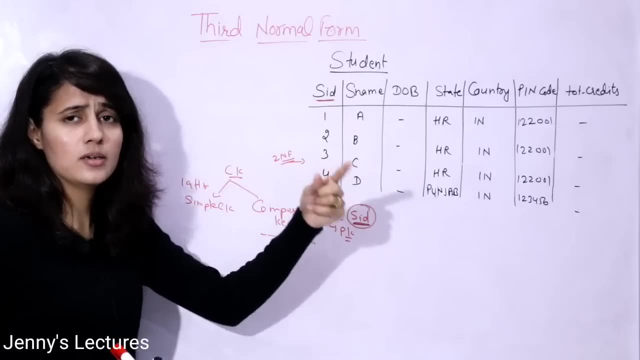 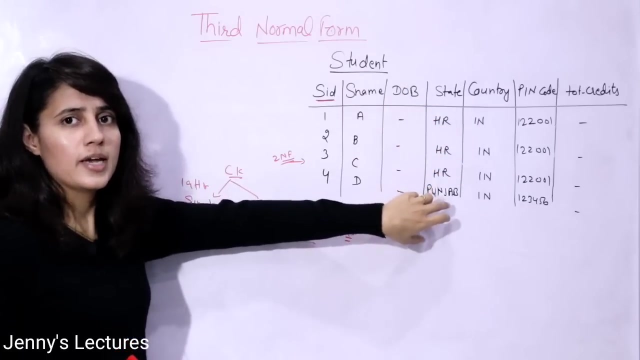 that relation would be in second normal form. Now why so? Because in second normal form there should be no partial dependency right And obviously it is in first normal form. it should be in first NF Student ID. that given relational table would be in first nf. so, and by looking at this table also you can see: 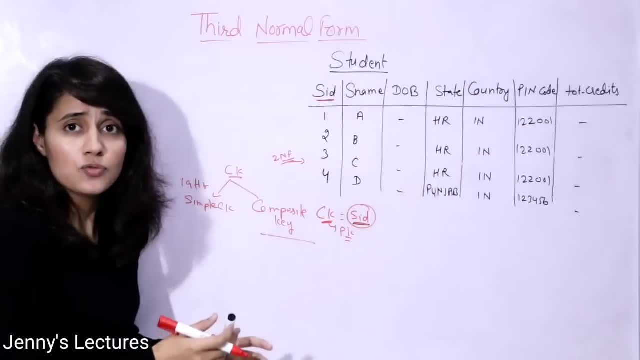 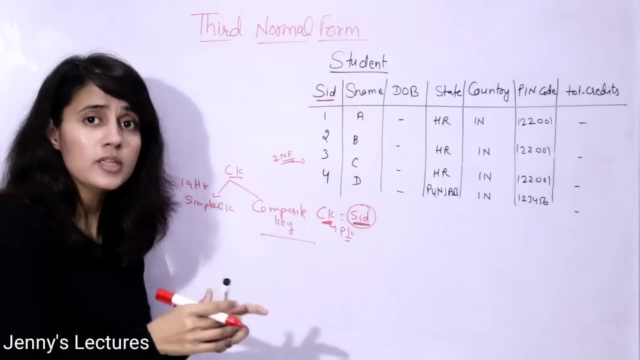 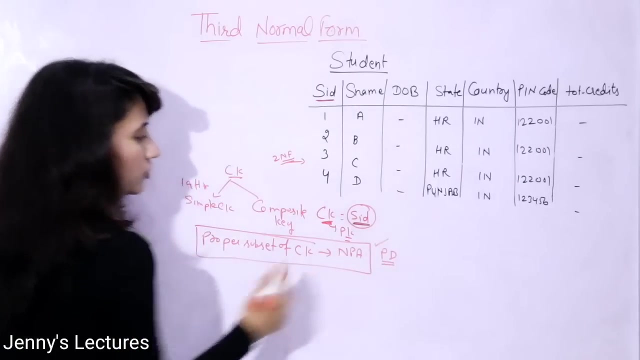 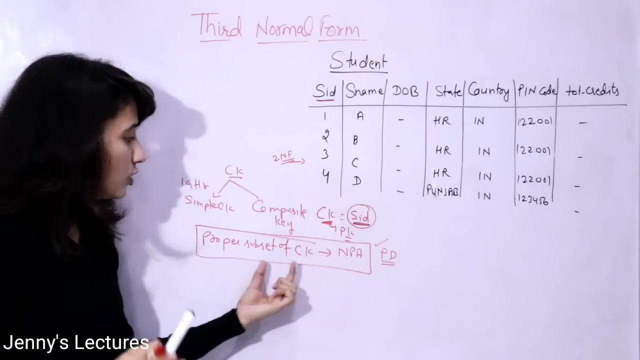 this is in first nf. now, partial dependency is what? if proper subset of candidate key determines known prime attribute, then only that is partial dependency, right? this condition is only of prime. sorry, partial dependency. this is the case here. proper subset of candidate key, this side known prime attribute, right? it's not like that. it is proper subset of candidate key and 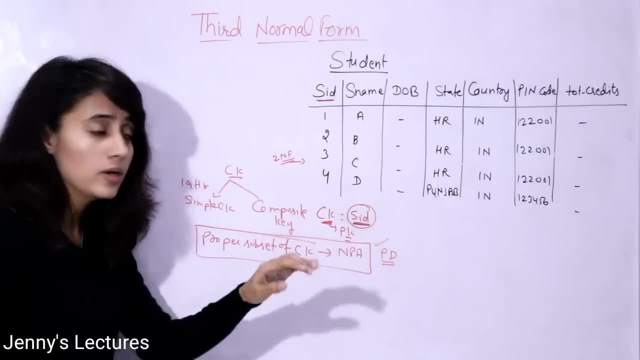 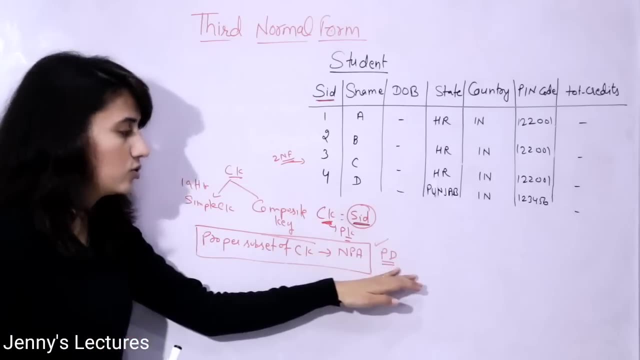 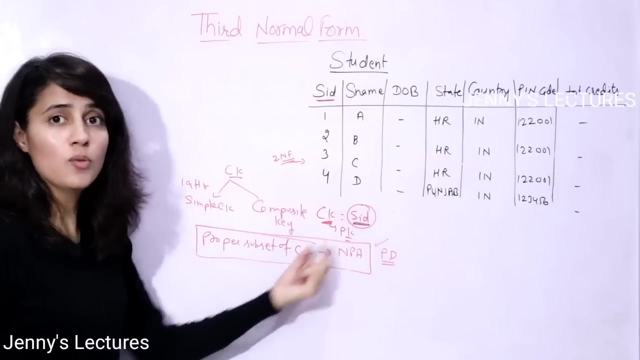 here we have prime attribute, then also partial dependency. no left side should be proper subset of candidate key. right side must be known prime attribute, then only it is known as partial dependency. now, if only one attribute is there, then obviously no proper subset is possible of this candidate key. if no proper subset is possible, then we will never get this kind of. 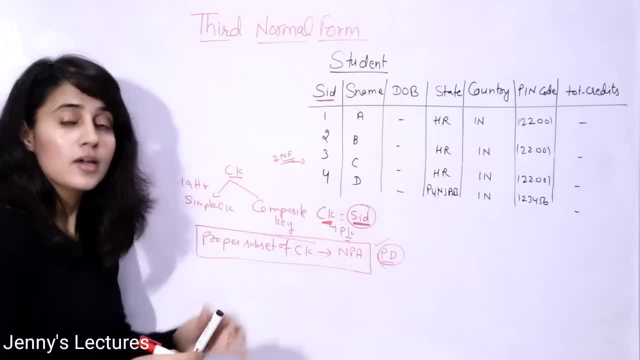 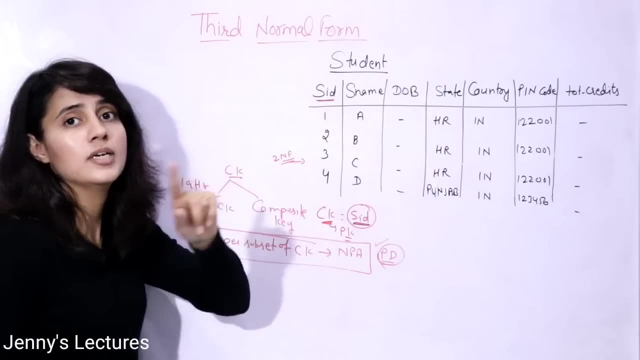 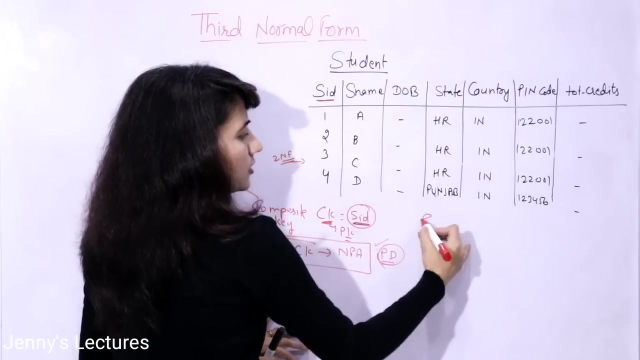 partial dependency here. so this is in second nf, right. but still, what can be the problem in this table if your database is in second normal form? that is also not considered as a good database. why so? because see here what you can say here the functional dependency is see: using pin code i can determine state and country. 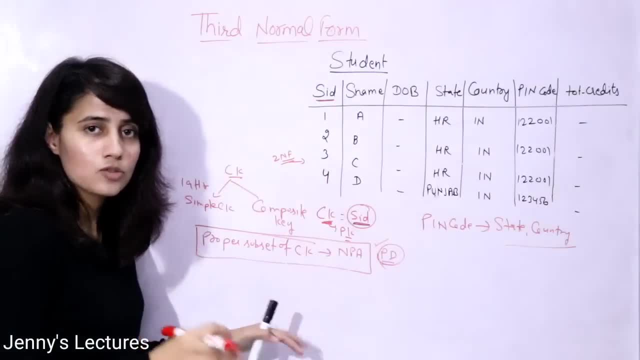 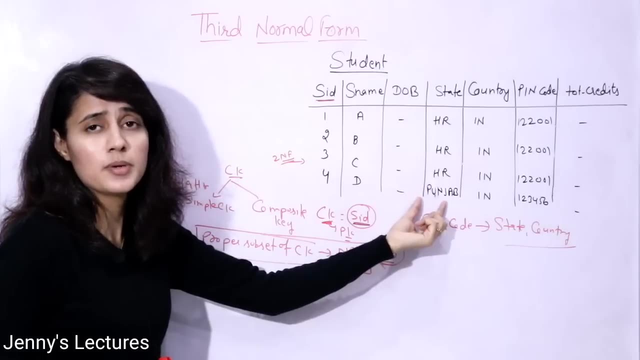 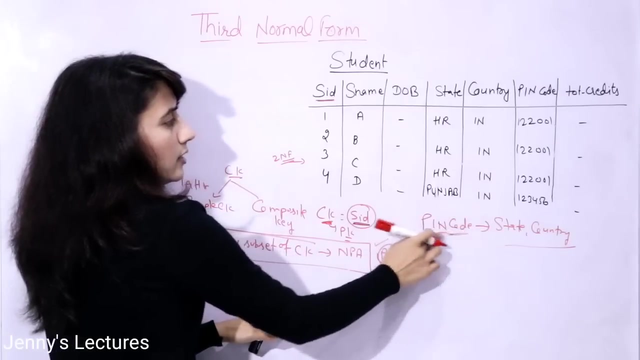 right. so this is the functional dependency present here and how to check that a particular functional dependency is valid or not, that also we have discussed in the previous video. you can check out that video in the cyber button right now. so and pin code- and the pin code is not any key here, no, cannot candidate. 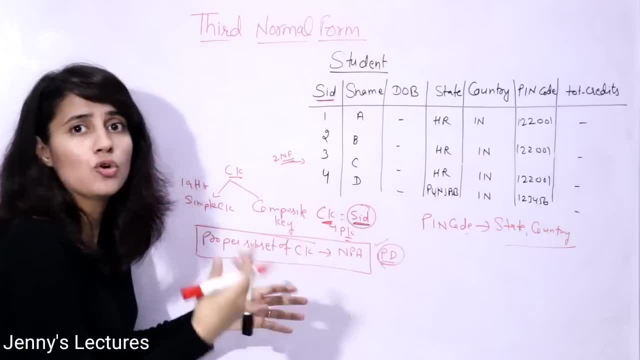 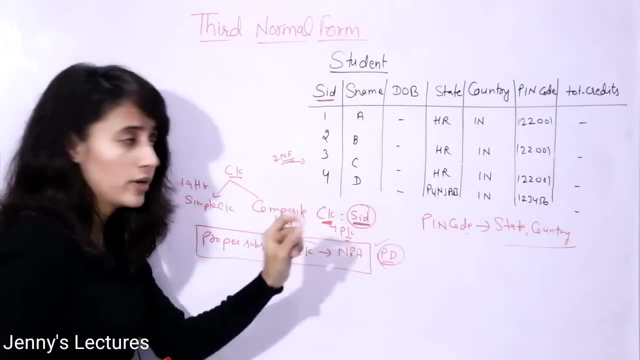 key here, right it's. if not candidate key, then it is known prime attribute. right, state and country are also known prime attributes. known prime attributes are those which are not a part of any candidate key. so here the prime attribute is only s id, because it is only 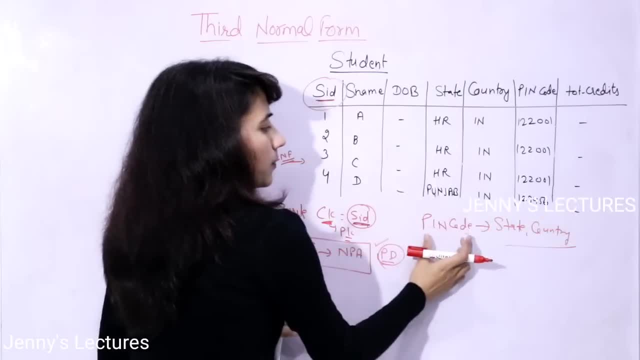 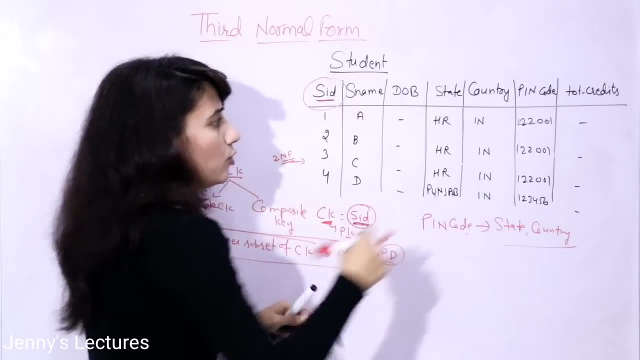 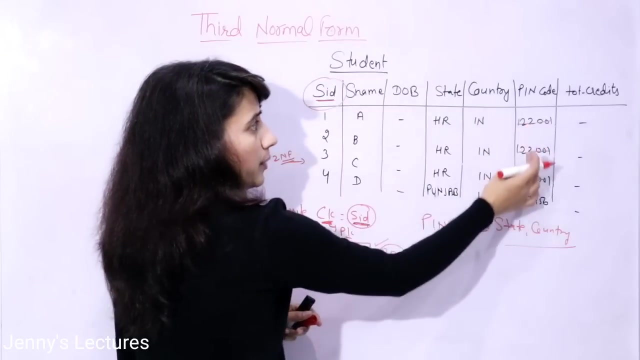 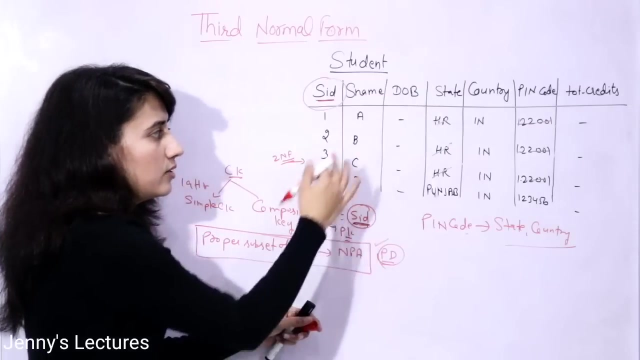 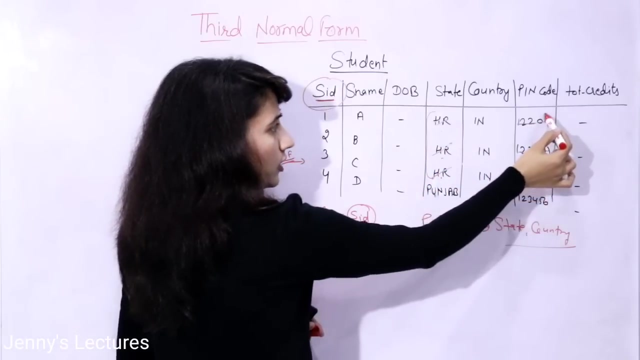 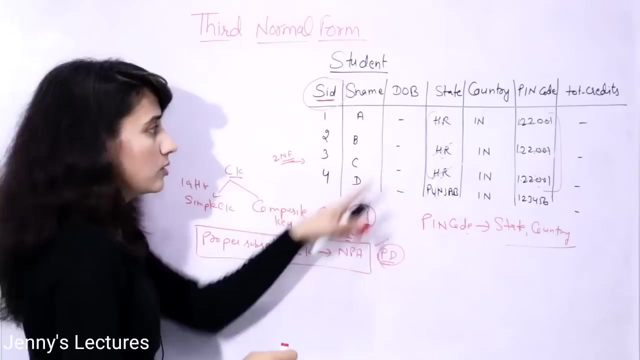 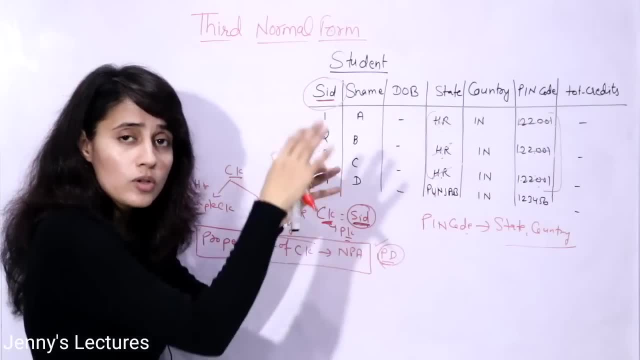 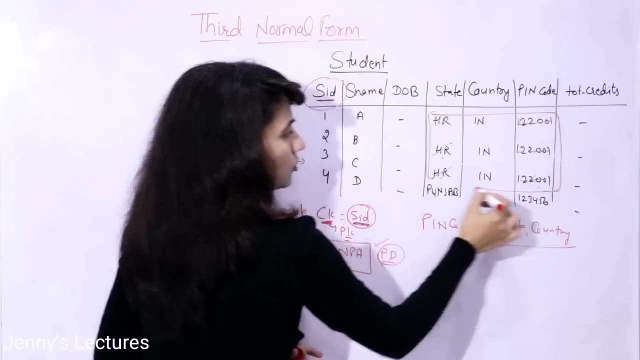 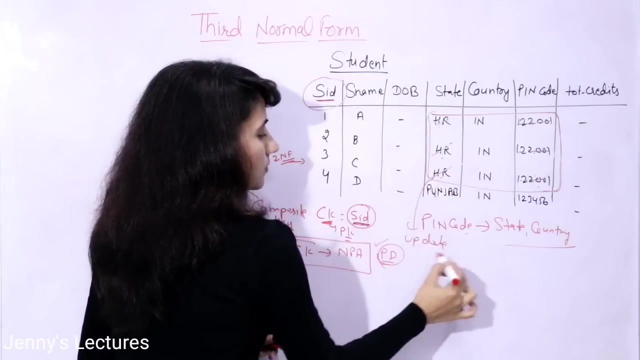 this situation is in 500 rows, so in all the 500 rows you need to update this change, right? this is what a redundancy. here you can see. this is what redundancy, right? so here you can have update anomalies. we have already discussed what are three anomalies: insert, update and delete. 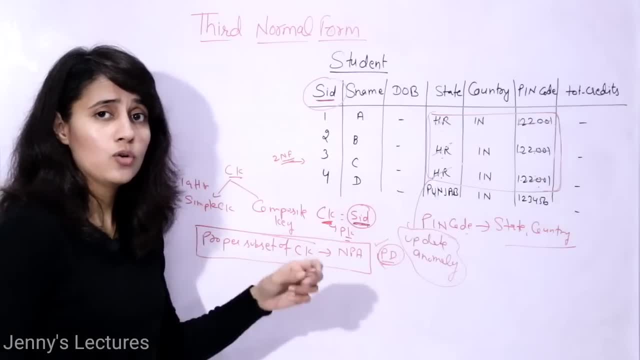 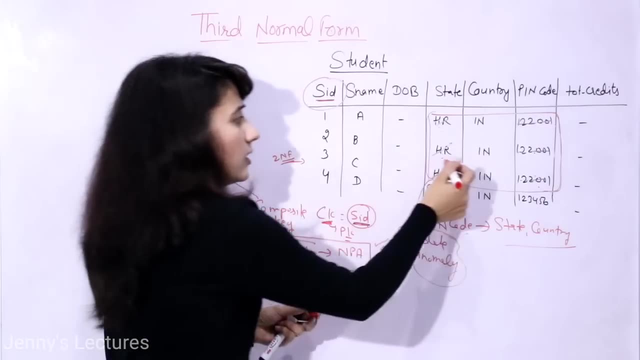 in the previous one of the previous video. right i will provide you the link of the complete playlist of dbfs in the description box. you can check out all the previous videos right. so because of this redundancy, we have update anomaly here. although the table is in second nf, still there are some. 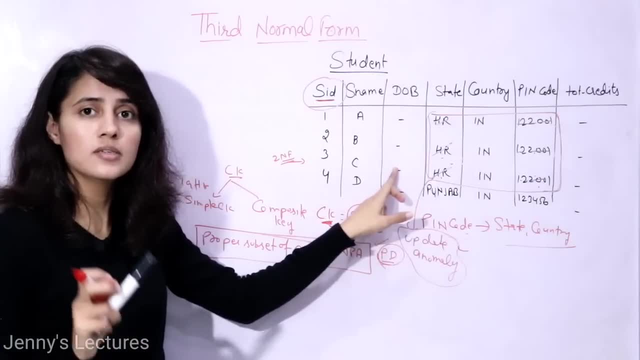 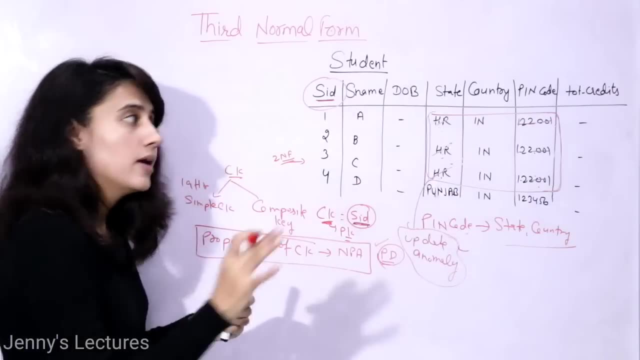 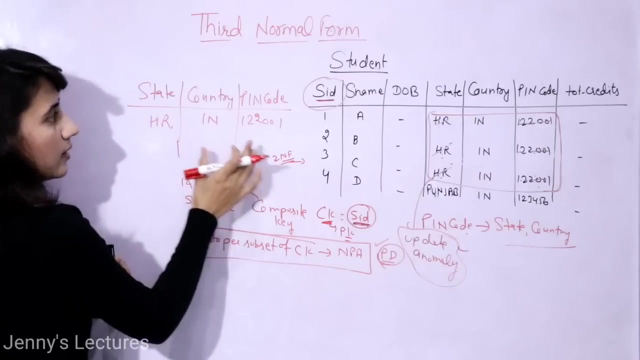 redundancy. still, we have update anomaly if table is in second nf, so to remove this one. what you can do, you can divide this table right in two tables. another table you can make which contains state, country and pin code, like this: this is the second table i have. i have taken this dependency. 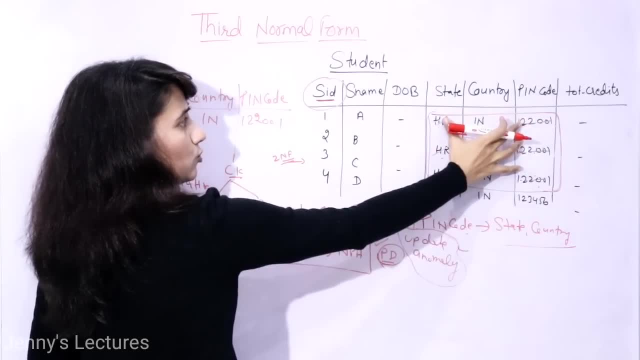 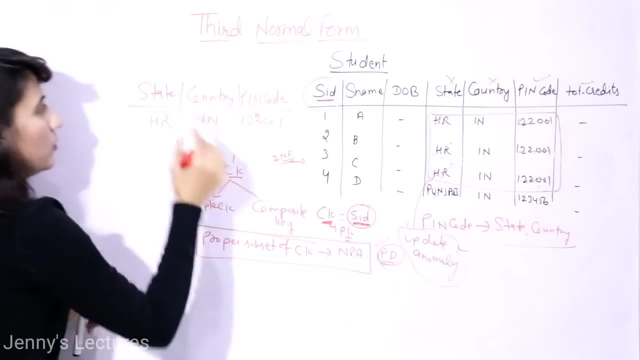 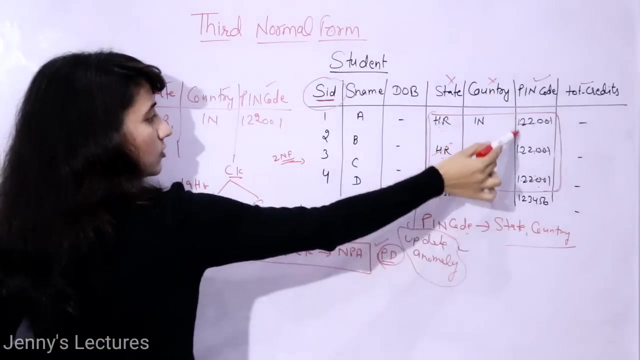 right and i have decomposed this table into two parts. one table will contain sid s name, dob, pin code and total credit note state and country. another table will contain state, country and pin code. right. so now, if you will change the pin code here at the three place, 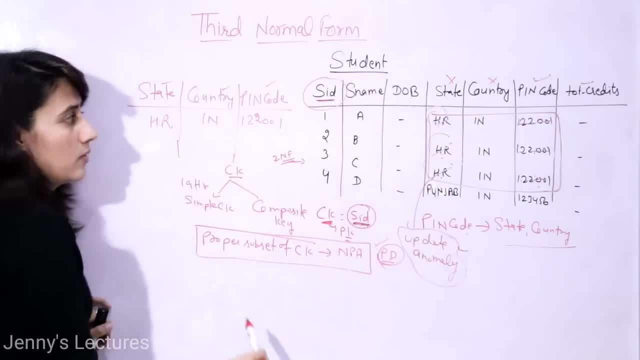 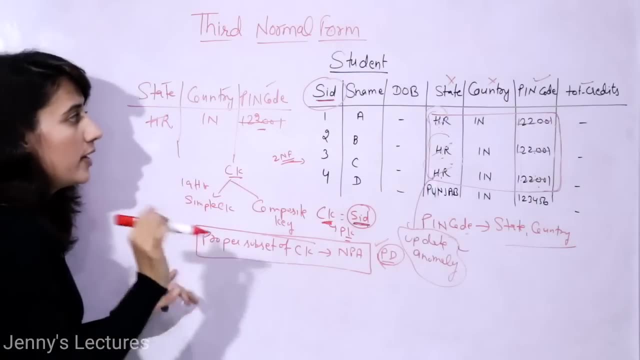 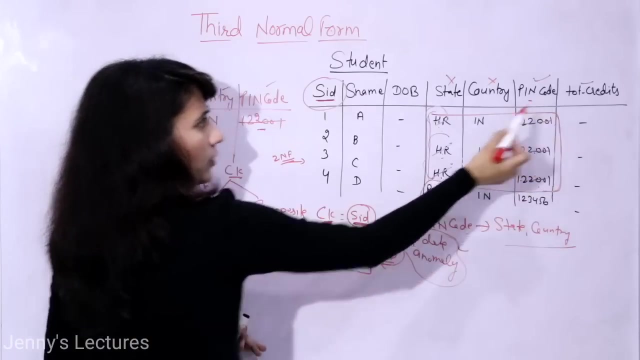 you need not to change that state at the three place right. only you can change here, one at one tuple, and here only you can change the state right. so now, here we have removed this redundancy, redundant data. although in one column, obviously, we have this pin code, we have to link these tables using foreign key. that also we'll discuss. 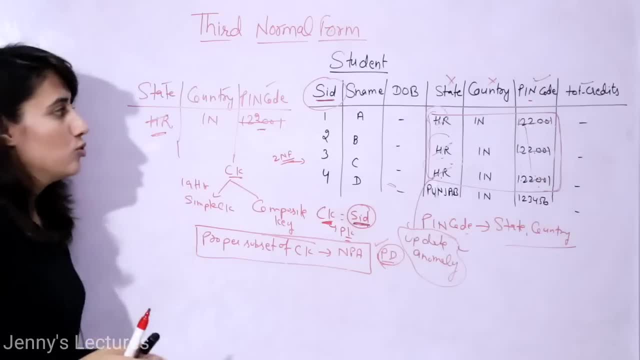 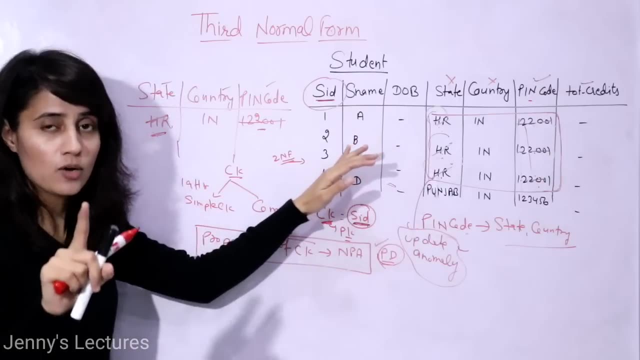 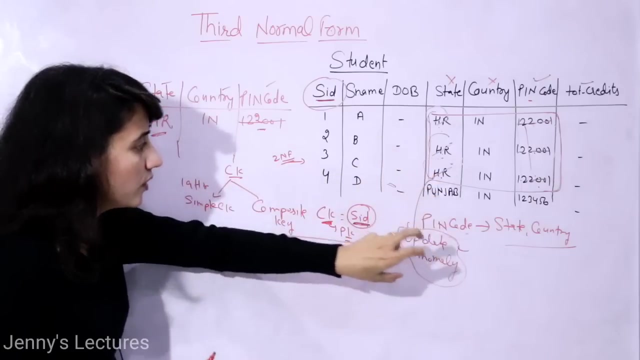 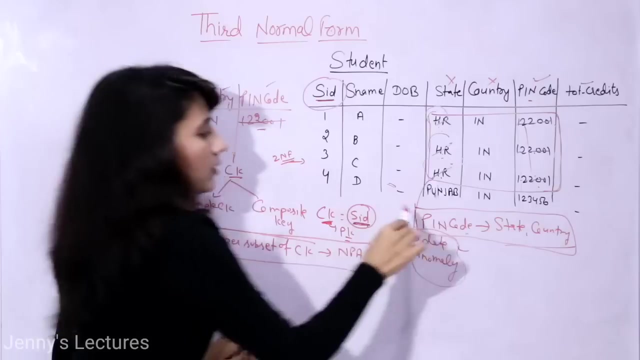 later. i'm just giving you a overview here. so now we have removed the update anomaly. now why this problem comes. see now- this is very important point- why this problem comes. obviously because of redundancy. but because of redundancy what? what functional dependency is there? because of that it the problem occurs because of this functional dependency, because 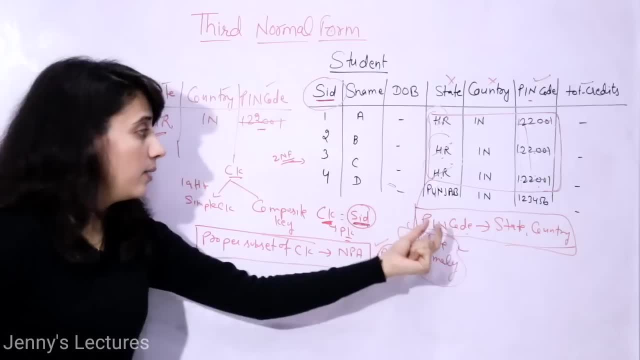 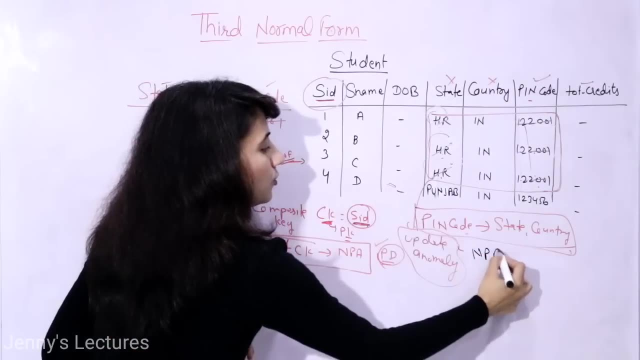 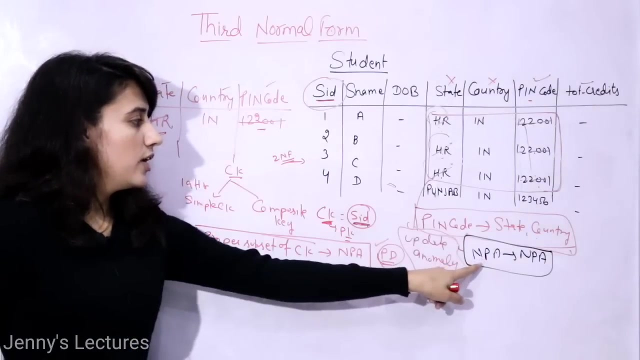 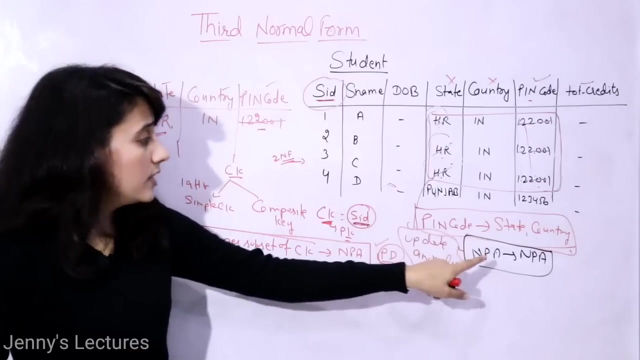 here pin code is determining state and country and pin code is known prime attribute, state and country. also known prime attribute. known prime attribute is determining state and country. meaning known prime attribute right. so this functional dependency, this type of functional dependency caused the problem here. you have to remove it. remove that and this functional 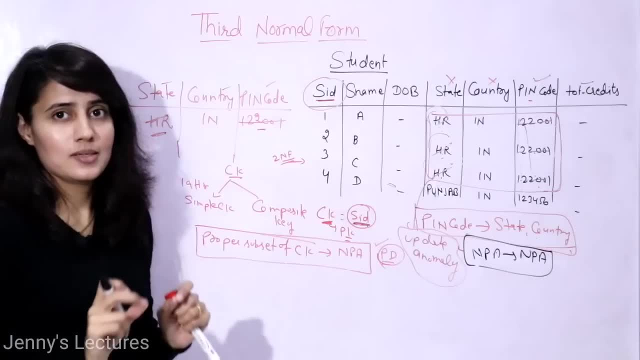 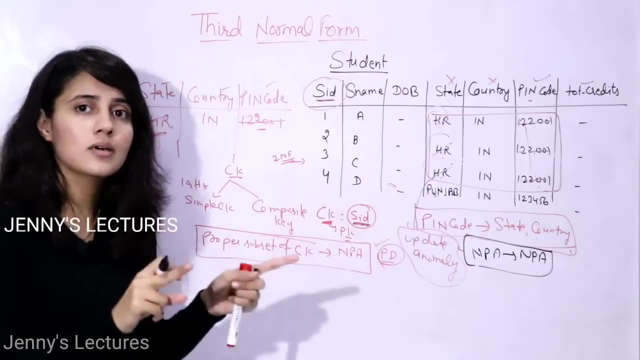 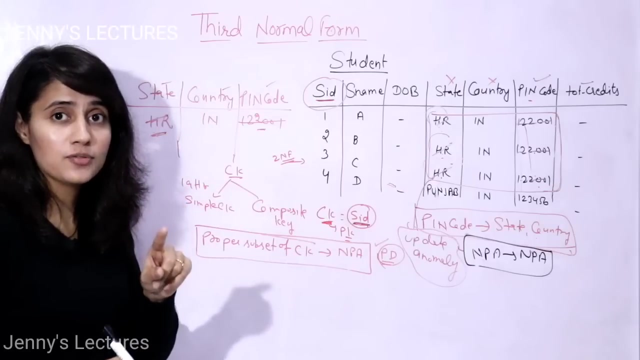 dependency is known as transitive dependency. right, if transitive dependency is there in the table, then that table is not in third normal form. so now, how can you, how can you say that our relation is in third normal form if- and only first one- it is in second normal form, that is for sure. second point is it does not contain. 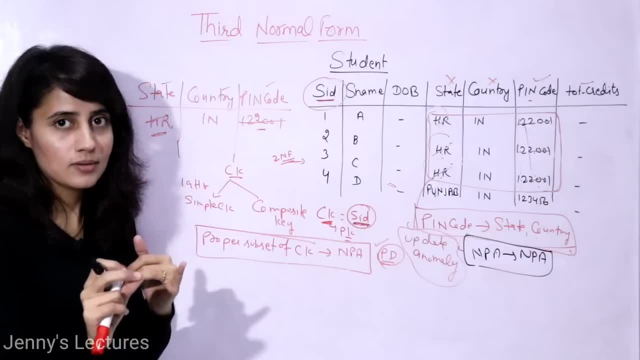 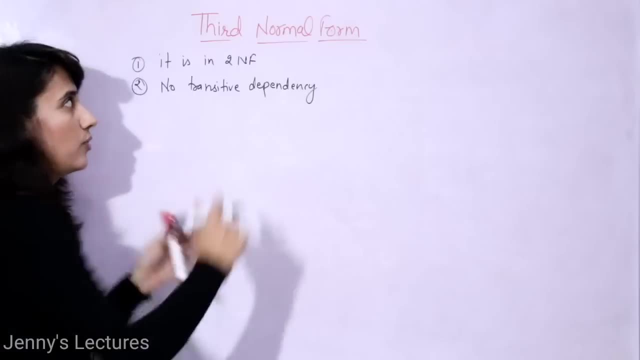 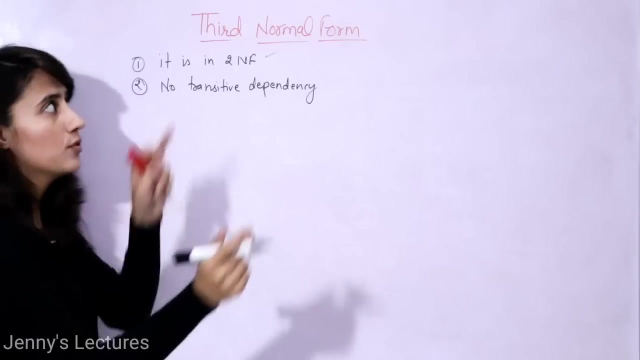 any transitive dependency right. two points are there. let me write. so these are two conditions for a relation to be in third normal form. first one: it should be in second normal form. you can say a relation is in third normal form if, and only if, first one it is in, it is in second normal form. 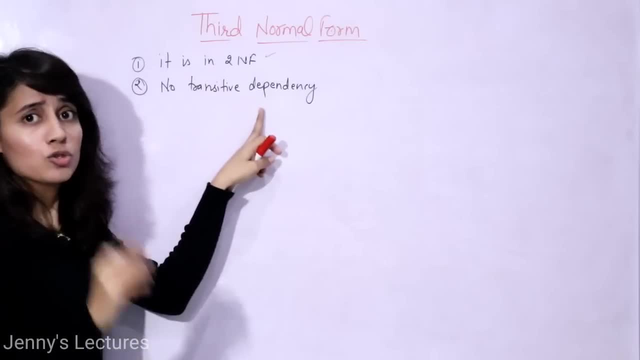 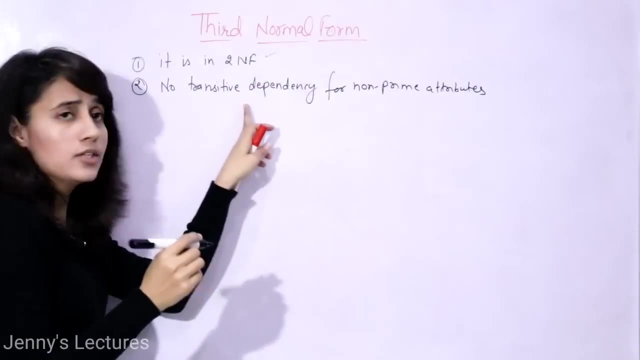 second one is: and only in third normal form. if a relation is in third normal form, an. if no, which means it? it means that there is no transitive dependency. or specifically, you can say: there is no transitive dependency for known prime attributes right now. what is transitive dependency? 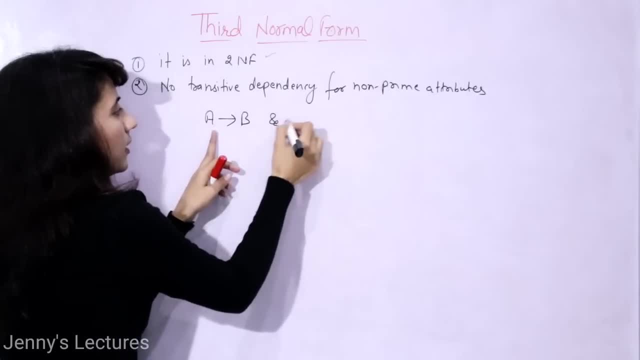 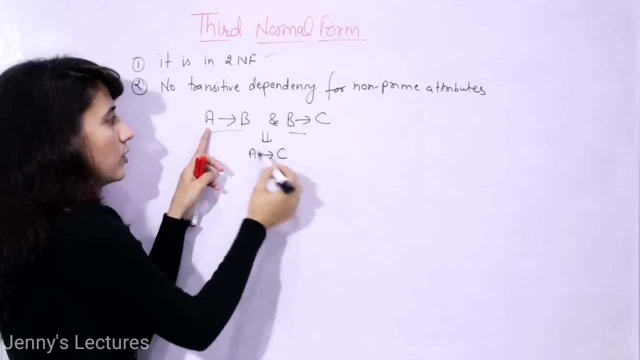 see if a relation, in a relation we have, a determines B and B determines C. right, so this is transitive dependency, because if this and this is given, you can say that A will determine C. this is what obviously you know. this is transitive dependency right now here. A is also known for known prime poser p comments. here you are looking at see page Andt artist results at p, e and p2 at ч in p2, C test manually recalling questions for p graph or measure: coop bums on program Andton's N conjist 7004, which is recipe for proof that feature. 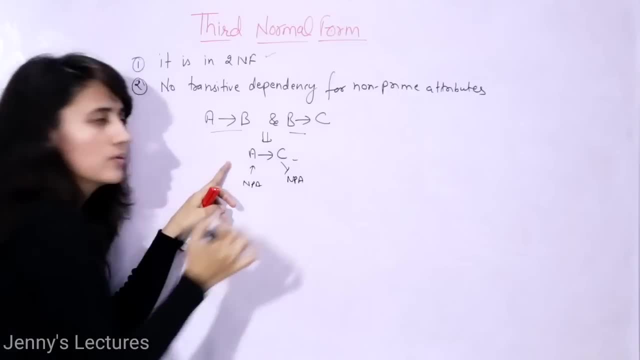 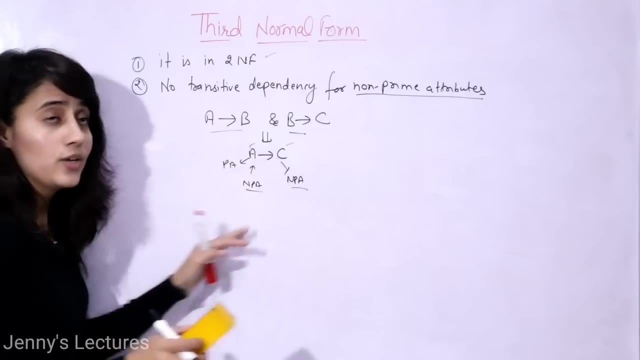 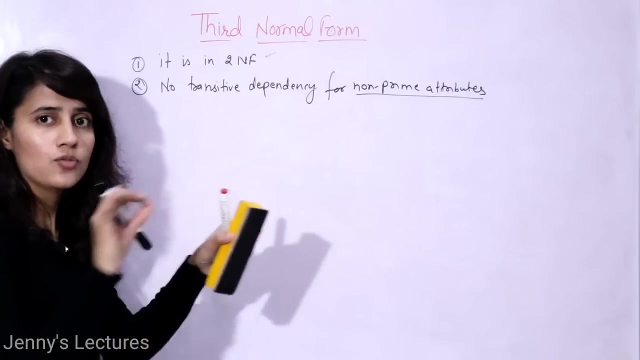 known prime attribute and c is also known prime attribute. if this is a case, then only you can say that in the relation we have transitive dependency present. so here, how can you write it if obviously they'll ask you in gate or net, so they'll give you one relation and set of functional dependencies. 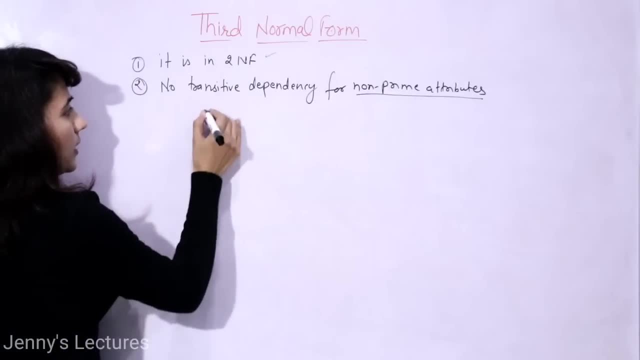 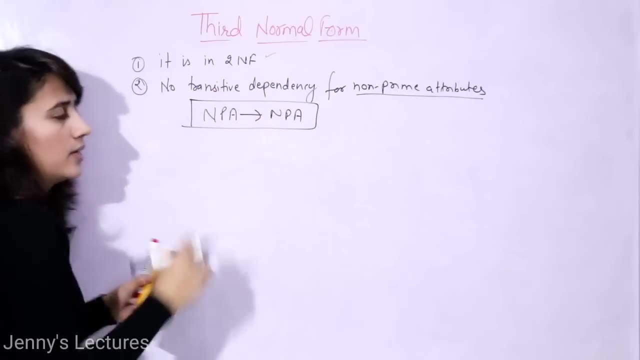 so if in the that set of functional dependency you find out a dependent dependency something like this: a non-prime attribute determining a non-prime attribute, then this is transitive dependency. it means that relation is not in third normal form. you have to check this only. 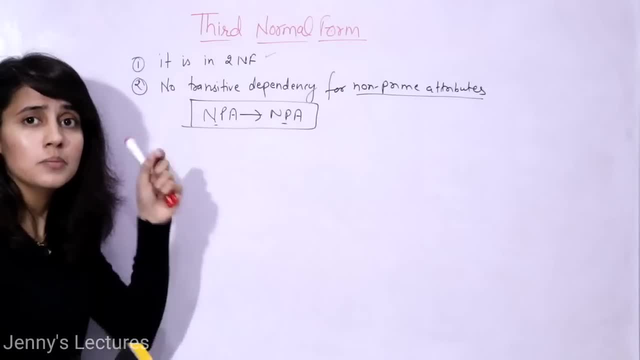 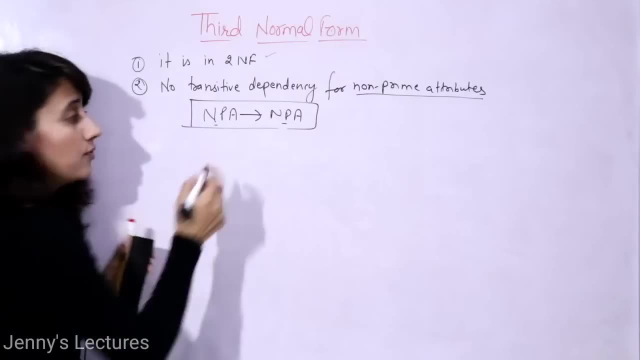 both side, left hand side and right hand side. both side must be known prime attribute. if any one is prime attribute then there would be problem. see, if this side is prime attribute and this side, this side we have known prime attribute, then this will create a problem for second normal form. 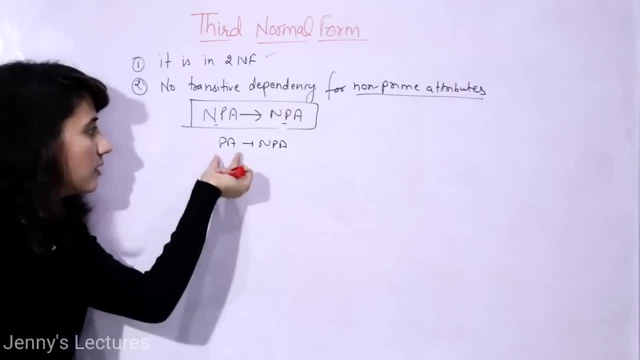 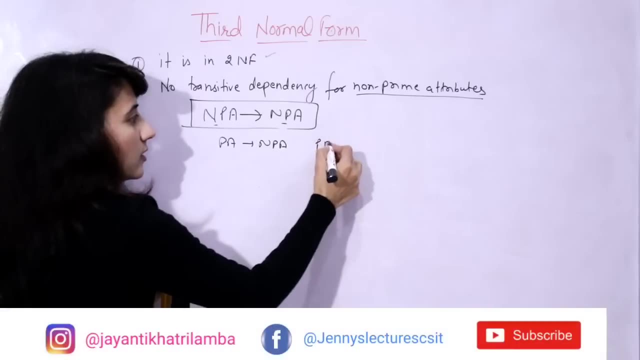 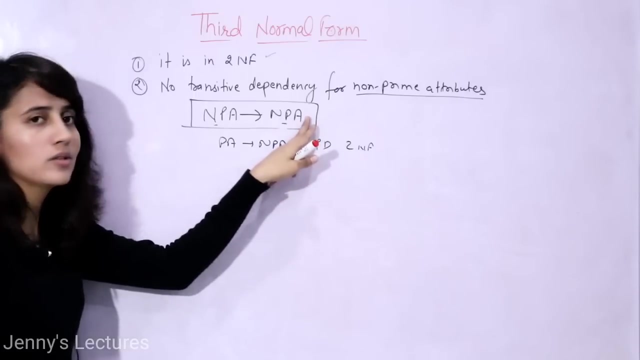 because this is what a partial dependency. if this side is a part of candidate key, right subset of candidate key, and this side we have non-prime attribute, then this has partial dependency. if this is the case, then that would not be in second normal form, right? so obviously, if not second normal form, then that is not in third normal form. 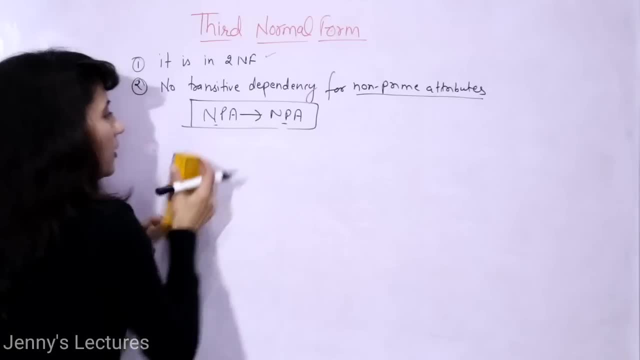 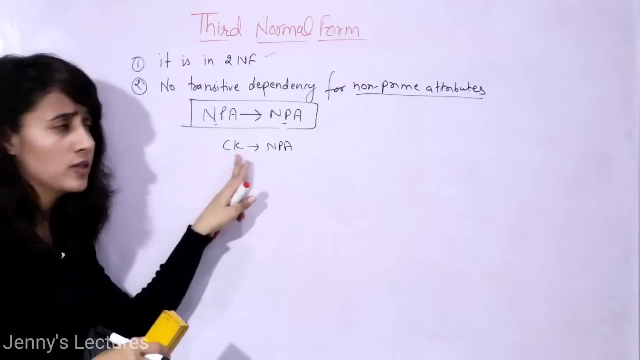 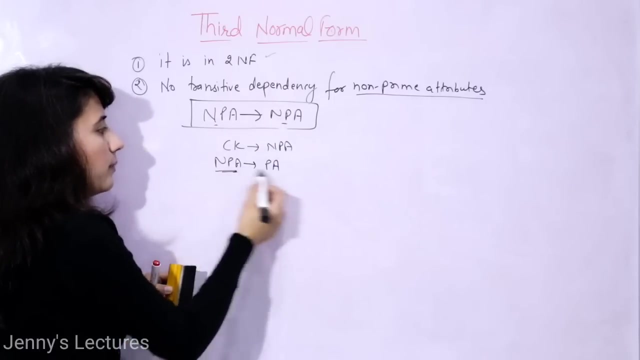 so now here, suppose, here we have candidate key and here we have known prime attribute, then that is, there would be no problem. this is not, you can say, a transitive dependency. and here suppose maybe you can get like this: here we have a known prime attribute and it is determining a 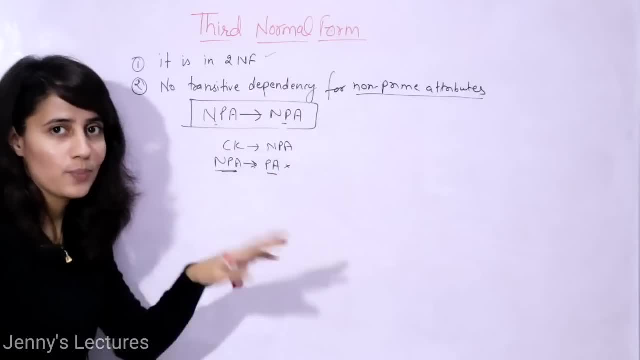 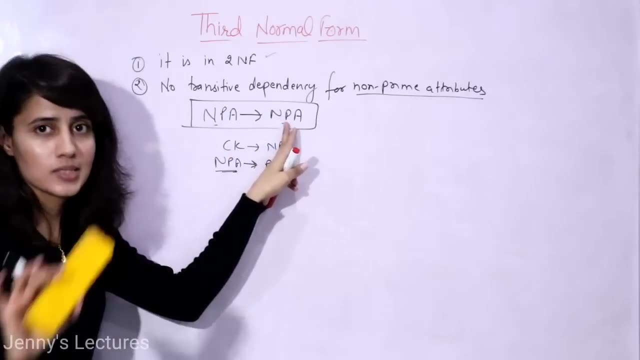 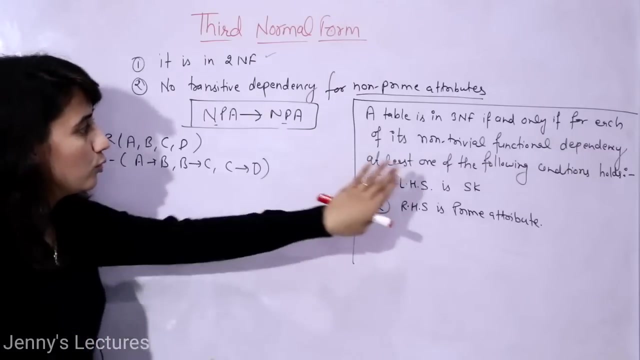 prime attribute maybe sometimes. then this is also not transitive dependency. for transitive dependency you must check both side must be known prime attributes. that's it right now. let us take one example now. let us consider this example now, before that. see, you can also write down like this: 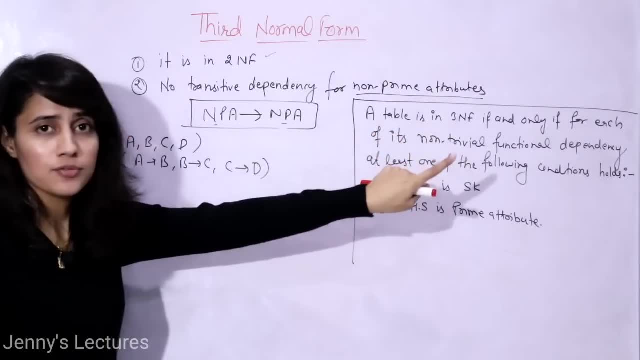 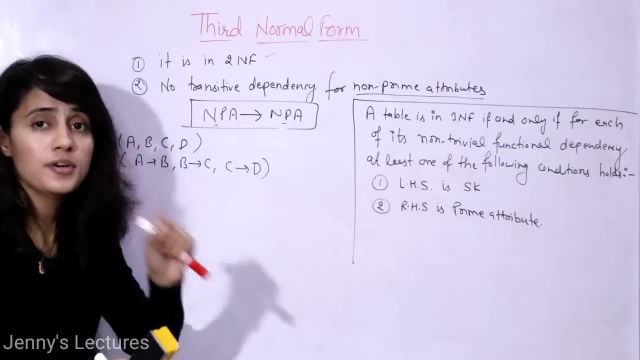 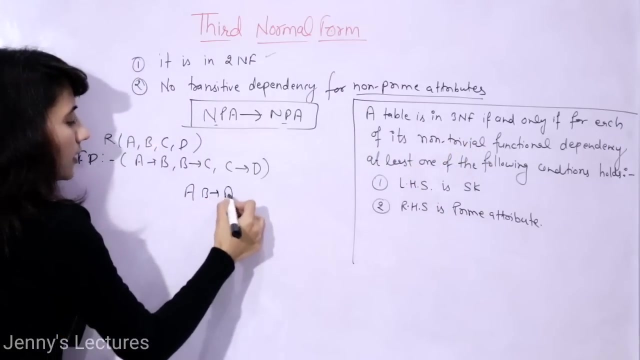 other table is in third normal form. if, and only if, for each of its functional dependencies right, and these functional dependencies should be known, trivial, for each of its known trivial functional dependency. if any functional dependency is given something like this: a, b determines a right, then we will not consider this case. for each known. 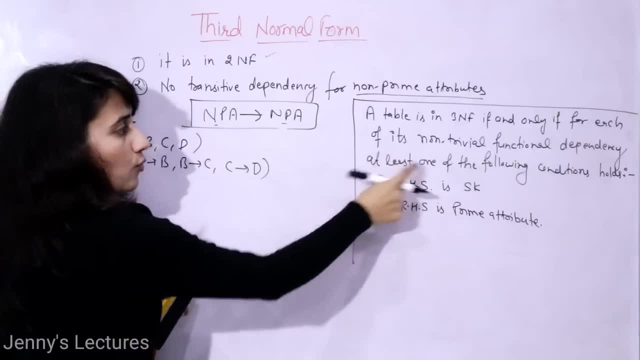 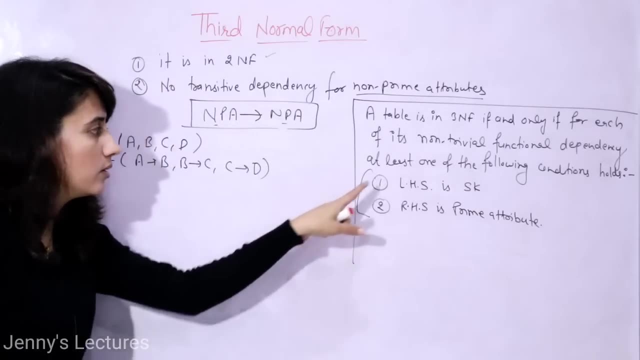 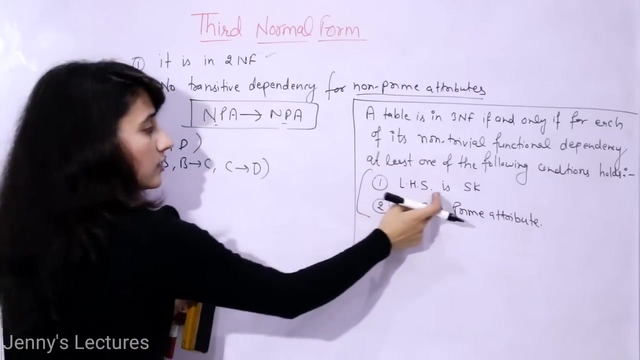 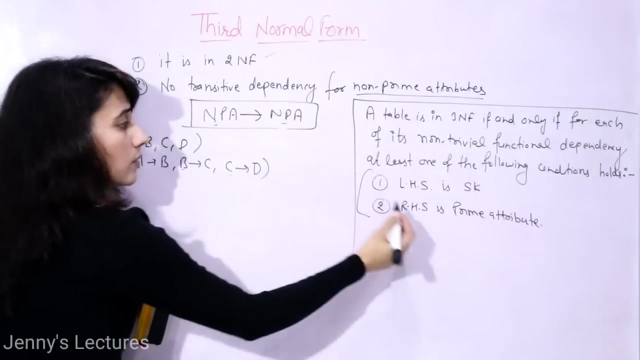 trivial functional dependency at least one of the following conditions hold. see, there are two condition, but at least one condition. it's not compulsory that these two conditions must be hold. in this functional dependency, at least one, either left hand side or right hand side, is super key. left hand side means this one right that determinant. or right hand side is prime. 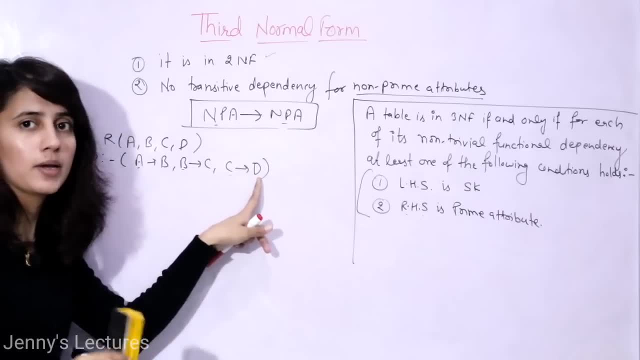 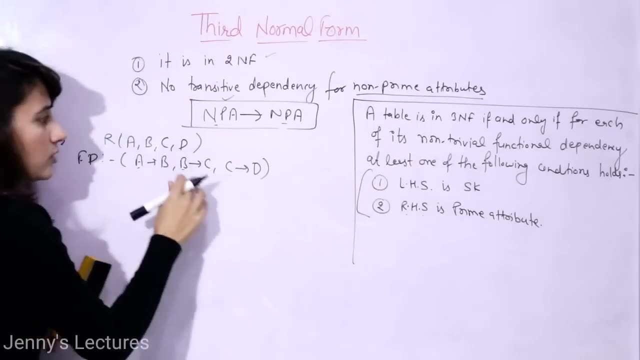 attribute means the dependent prime at is prime attribute, at least one of these conditions hold. you can write down something like this: or you can write down something like this for this: obviously for finding the known prime attribute. or you can say, for finding the super key or the prime attributes. 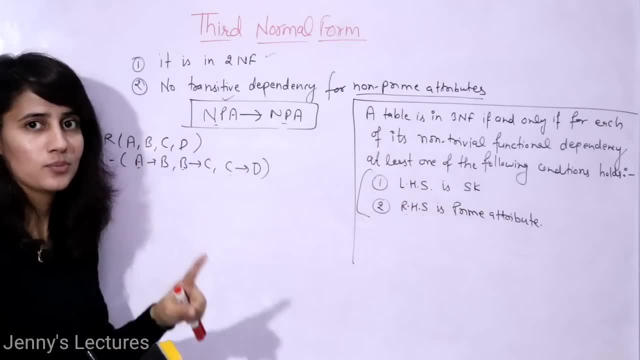 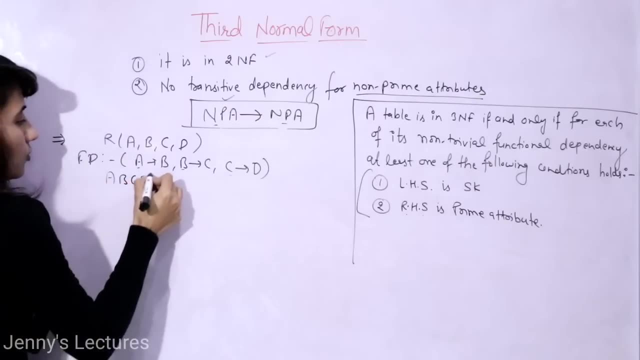 you must need to find out the candidate key. that is very important point that also you have discussed in one of the previous classes. i will explain in detail later. but now let us see what is happening here. previous video: right, how to find out candidate key. see a, b, c, d closer you can take all the 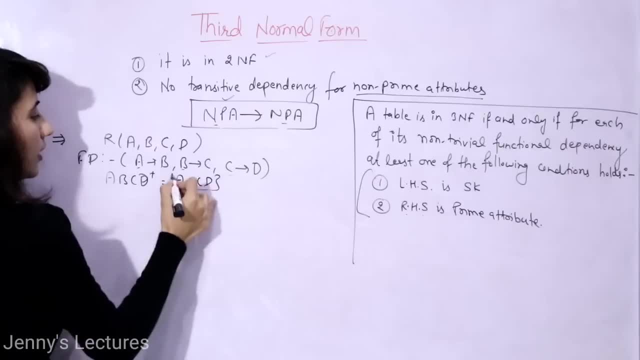 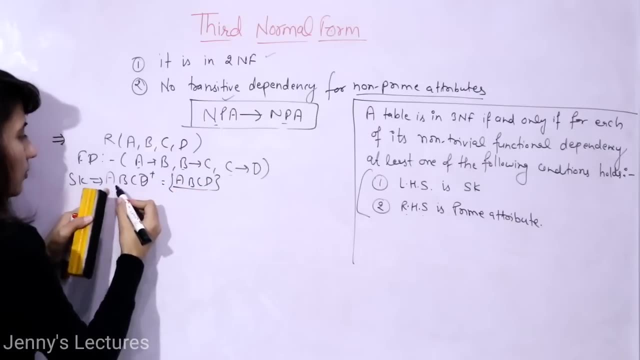 attribute first of all. definitely it will find out all the attributes so you can say that a, b, c, d is super key. now find out candidate key. try to discard the elements, the attributes here. see a is determining b, so you can discard b. a is determining b. b will determine c, so a will. 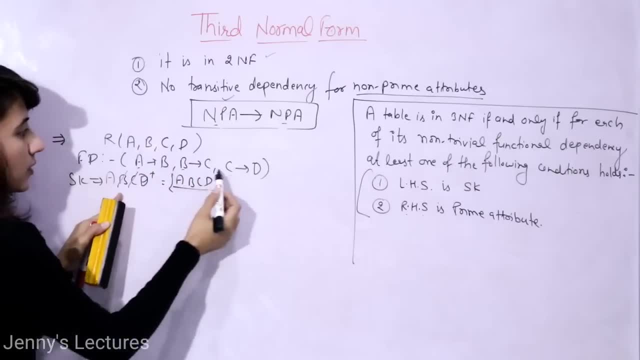 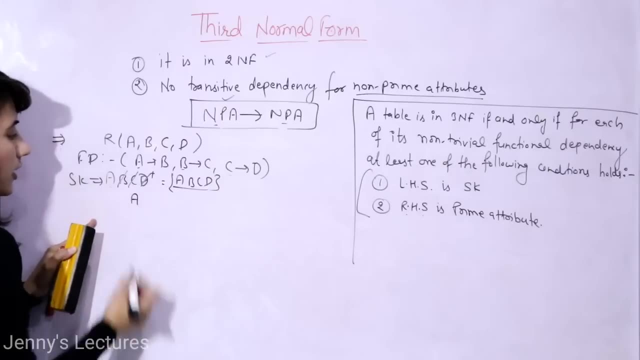 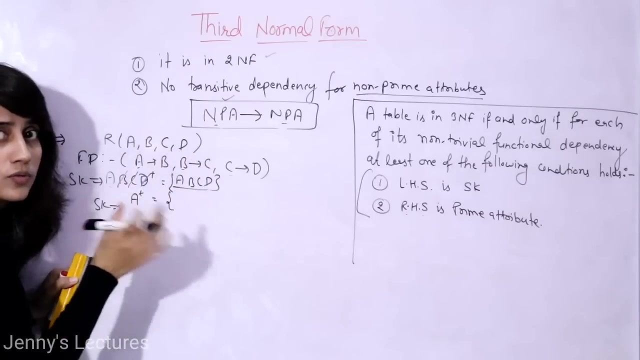 determine c, so you can discard c because we have a. c will determine d, so by transitivity property, a will determine d. we have a, so you can discard d. so we have only a. so a is what super key you can check. if the attribute closer of a is having all the attributes of the relation, then 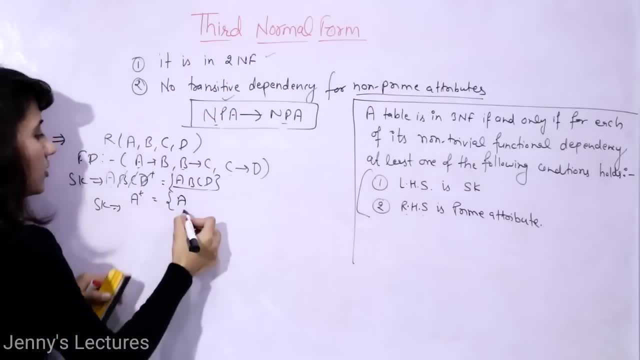 definitely it is. it is a super key. you can check a will determine itself right by reflexivity property p less like b. we have a, so i can determine b using b. i can determine c using c. i understand remind d, so all the attributes are there in the attribute closer of a. so a is what super key. 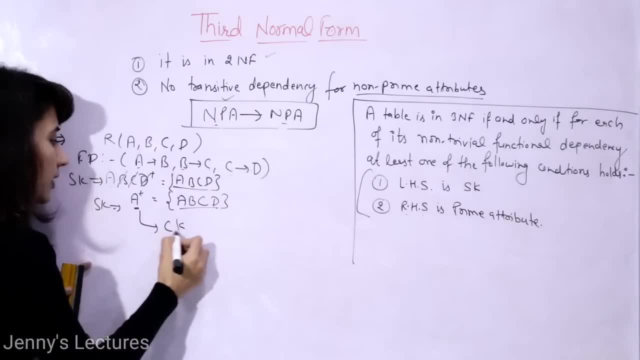 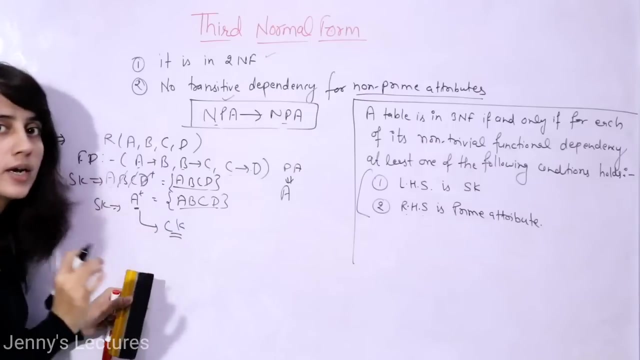 now as a candidate key. definitely a would be candidate key. why so? because no proper subset is possible of a is only single, having only single attribute right. so this is what candidate key now we have got, one candidate key, so means prime attributes we have got that is one that is. 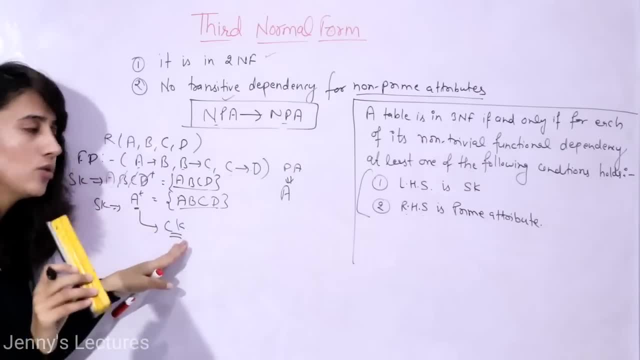 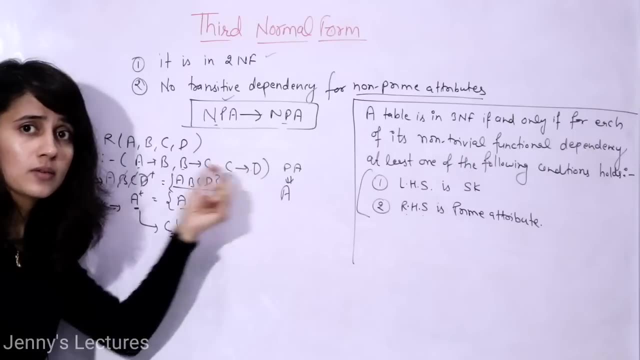 a now check out. more candidate keys are possible here or not in this relation. how to check out this thing? if the prime attribute is present at the right hand side of the functional dependencies, then definitely there would be more candidate keys and you have to find those out right. but 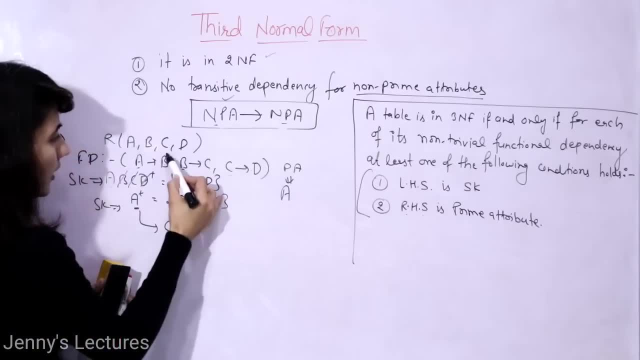 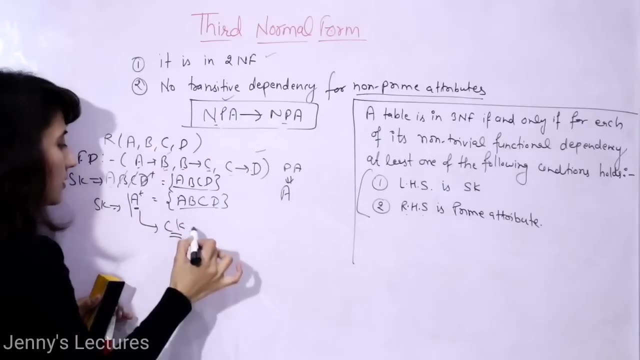 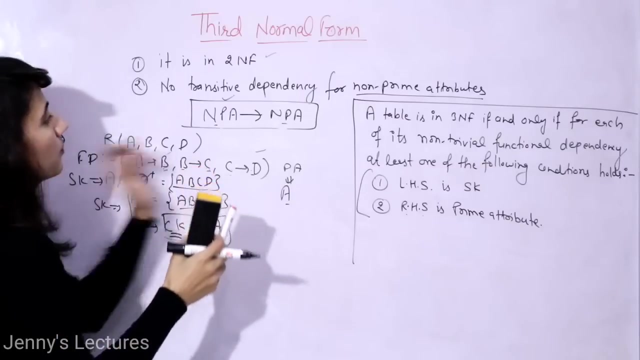 here. check: a is prime attribute. is a present on the right hand side? no, no, no. so now there is no more candidate key. now we have only one candidate key. that is a in this relation, right, and this is prime attribute. now you can check this condition, this kind of 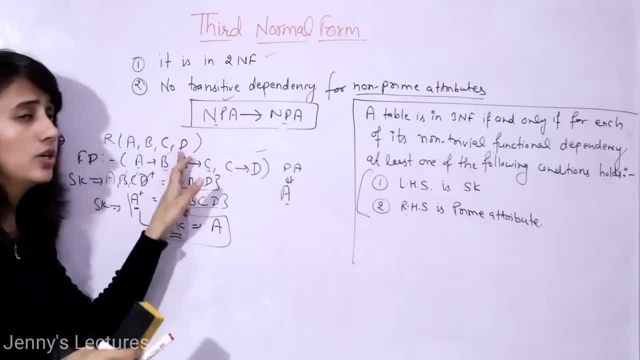 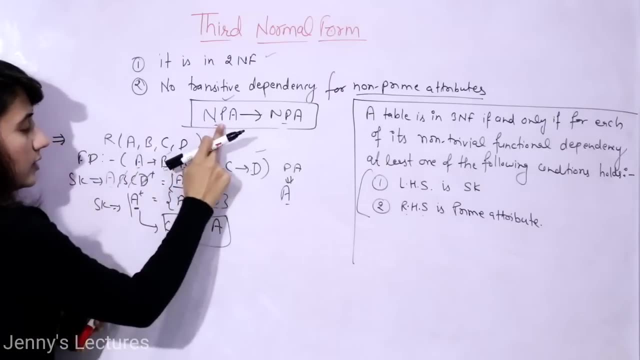 dependent key is present on the right hand side of the functional dependencies, then definitely there is a dependency present here or not? if yes, then this relation is not in third normal form right check out. check the first dependency: a is a non-prime attribute. no, it is prime attribute. so 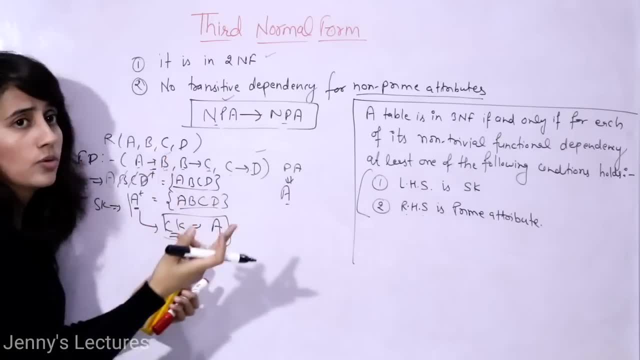 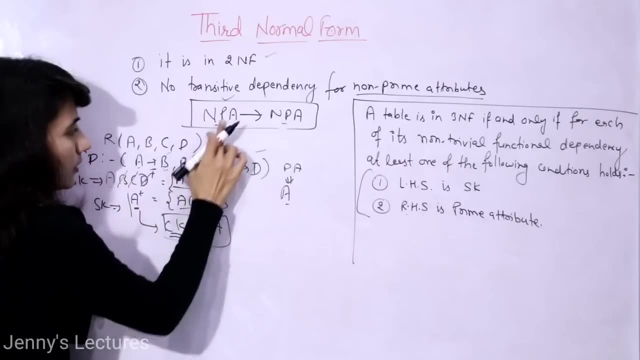 this is what this is not. we can say that this is a transitive dependency. no right, so this is not a transitive dependency. now check out this one b. yes, it is non-prime attribute, but only checking b. you can't say that this is transitive dependency. you have to check the right hand side of the. 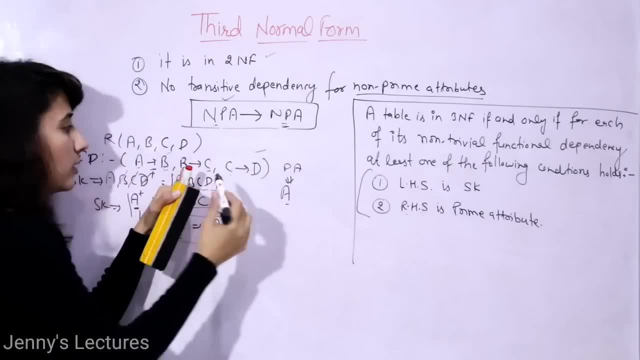 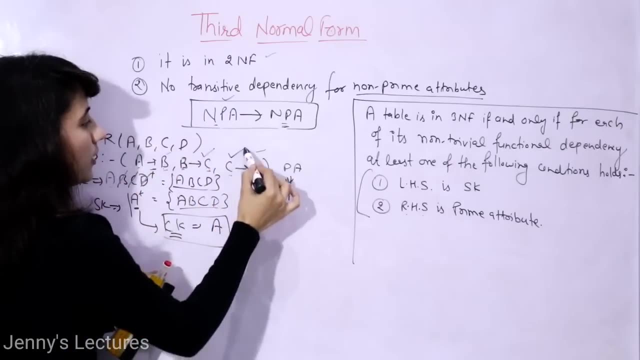 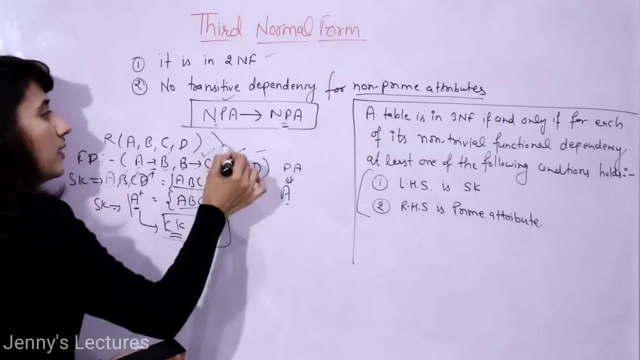 side also, because there also there should be non-prime attribute c. c is also non-prime attribute, so this is transitive dependency. c is non-prime attribute, d is non-prime attribute, so this is also transitive dependency. so two transitive dependencies are there, so this relation is not. 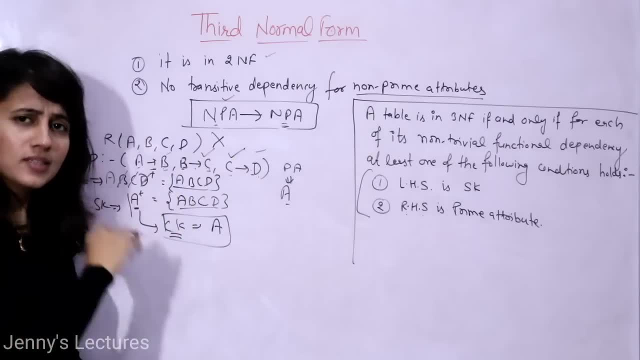 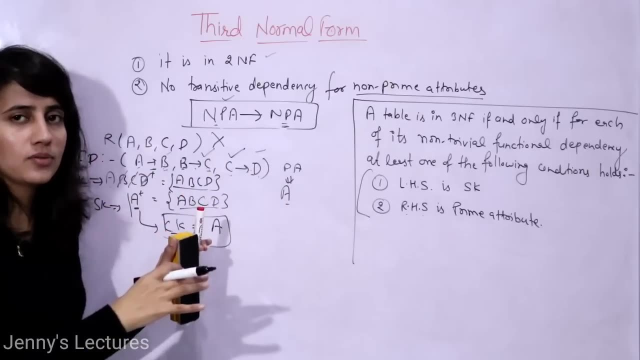 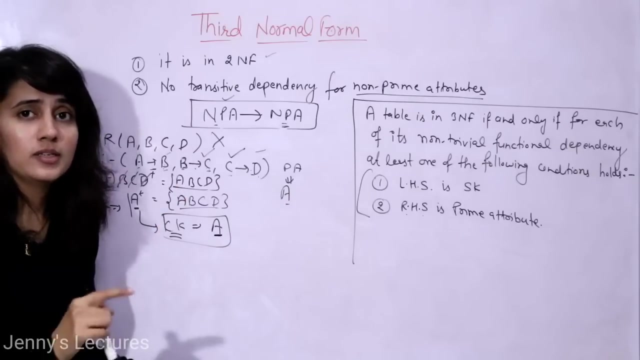 in third normal form. right, this is in second normal form because by default i have taken these type of functional dependencies uh, so that this is in second nf. you can check out this also because if candidate key is having only one attribute, then definitely that relation would be in second normal form. so this is also in second hand. sorry, not in third, but only second nf or here. 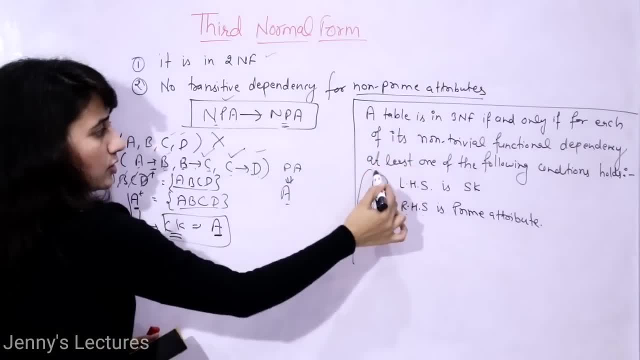 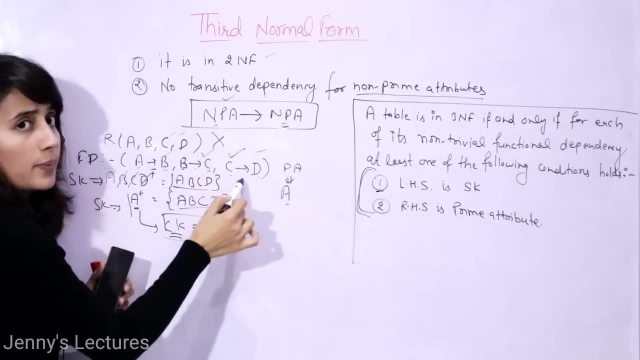 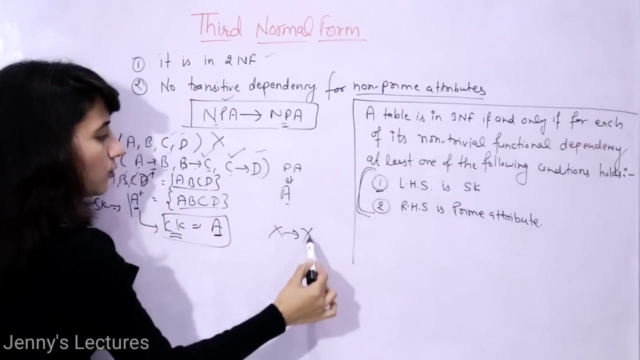 if you will not check like this, so you can check like this. check these two condition: first one is left hand side- is at least one condition must hold for each non-trivial functional dependency. see, these are non-trivial functional dependencies, right trivial. i guess you know that if x determine y, then 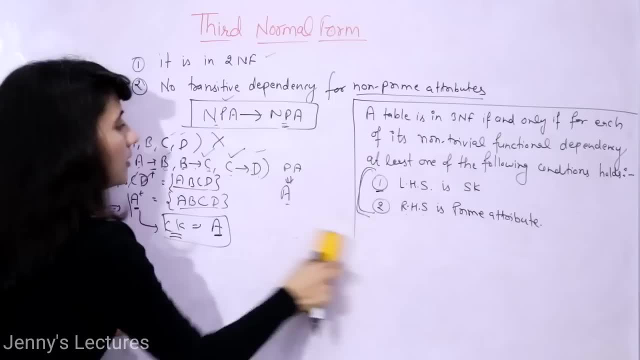 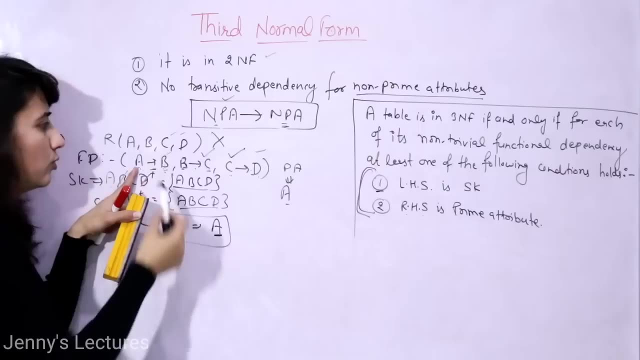 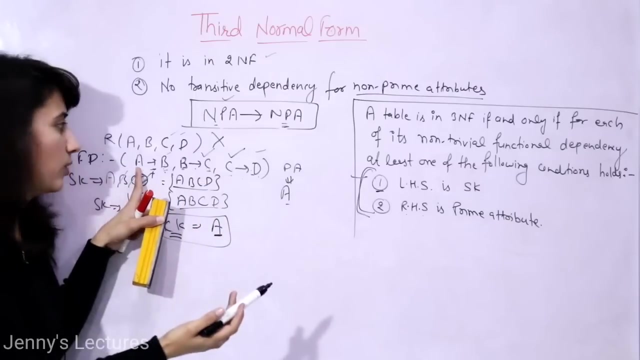 this is a trivial functional dependency. right now, see, left hand side is super key. check out for this one. left hand side is super key. yes, right, no need to check the right hand side. only one condition, at least one condition, must hold for the relation to be in third, normal form. 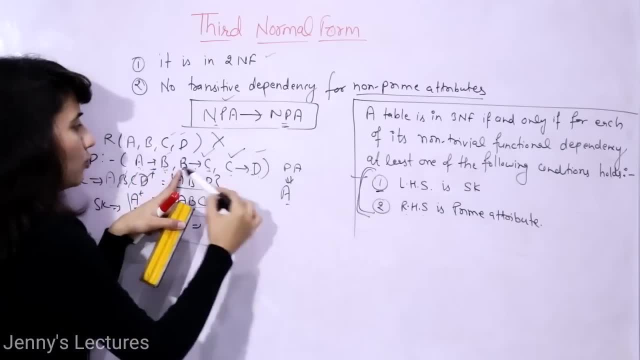 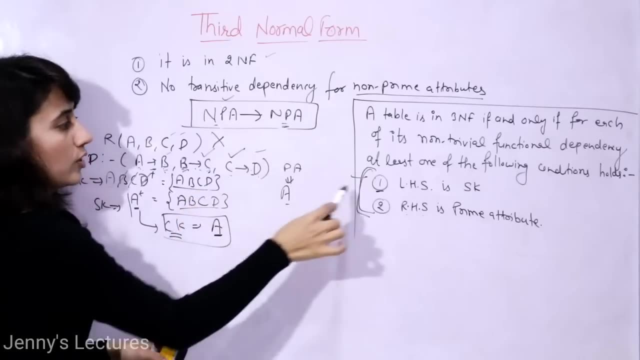 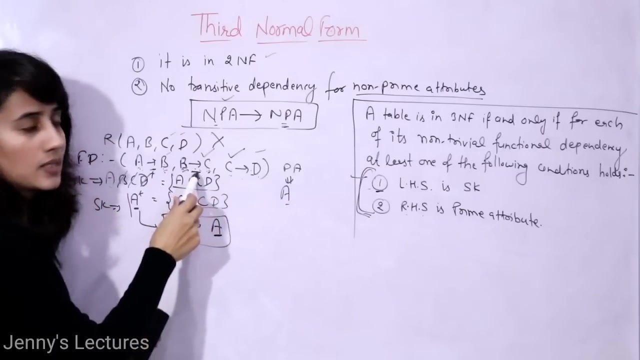 so check out for second functional dependency: left hand side. is it super key? no, b is not super key. now check for right hand side. right hand side is prime attribute. no, so neither this nor this one is present in this for this functional dependency. so this is transitive dependency. 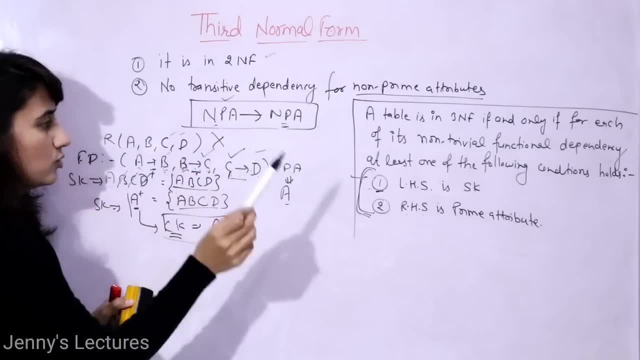 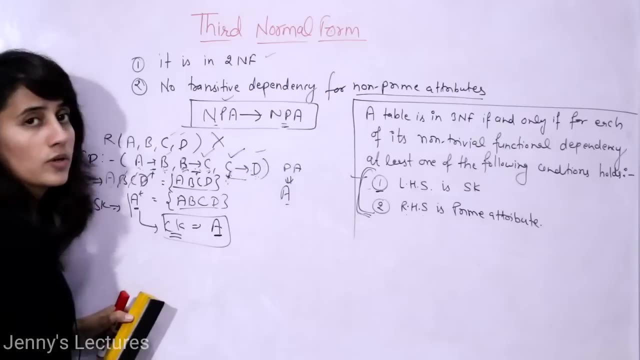 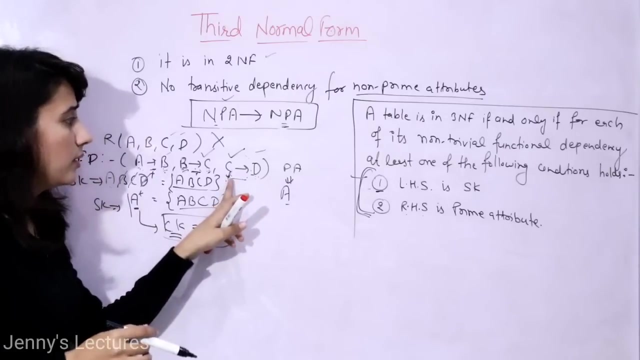 this is also because left hand side check it is super key. is it super key? no. so now right hand side, is d prime attribute. is the prime attribute? no, so neither this nor this one is holding here right now. it is also transitive dependency. see here why i am saying that c is not a super key. 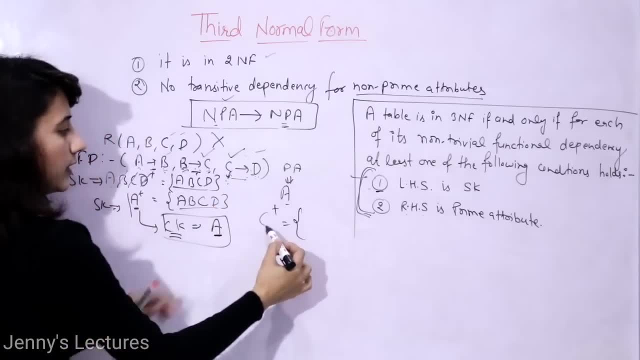 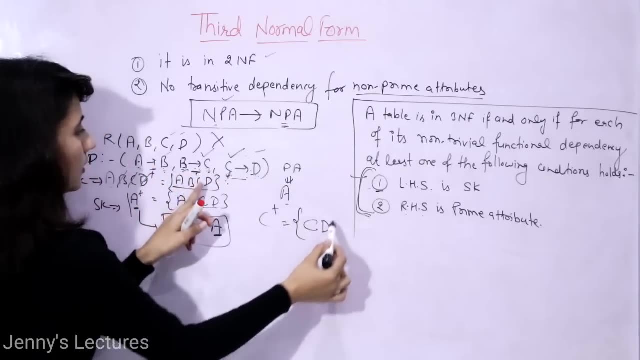 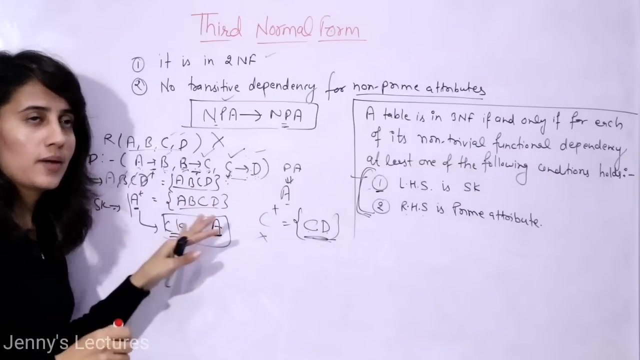 obviously, if you find out the c closer, then what it contains it will determine c itself by reflexivity property and using the functional dependency c can determine d, nothing else. so attribute closer is containing only cd, not all the attributes. so c cannot be a super key right now. let's take a different type of example. so let us take this example. here we have 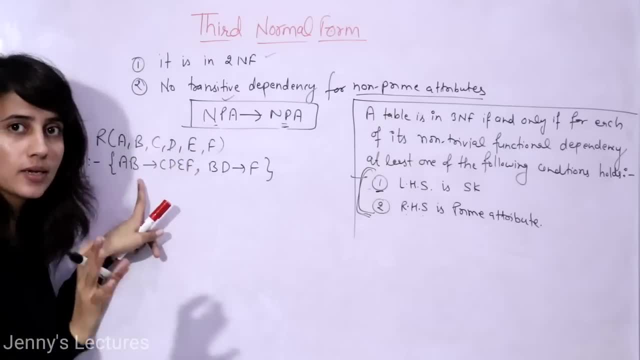 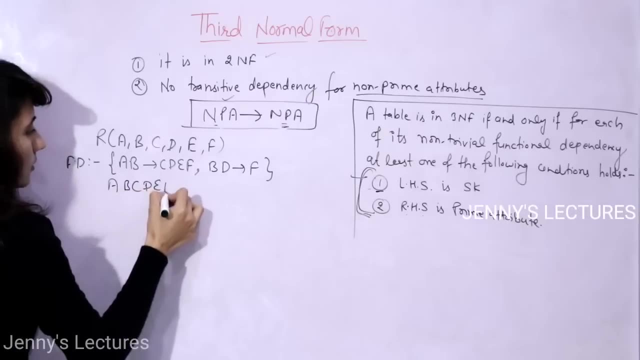 a, b, c, d, e, f attributes and these two functional dependencies are given right now. first of all, obviously find out the candidate key here. now, candidate key is this- closer would contain all the attributes. so this is definitely a super key. now try to discard the attributes from here. see the functional dependency: a, b is determining c, d, e, f, right. 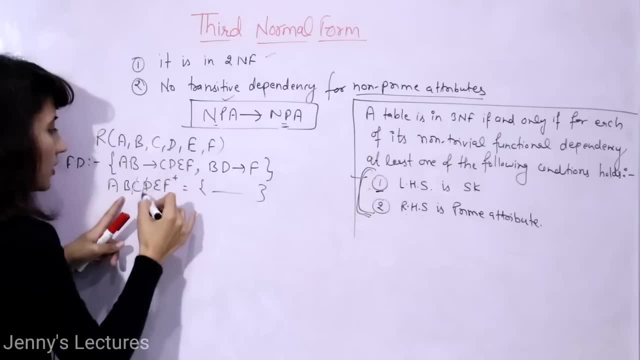 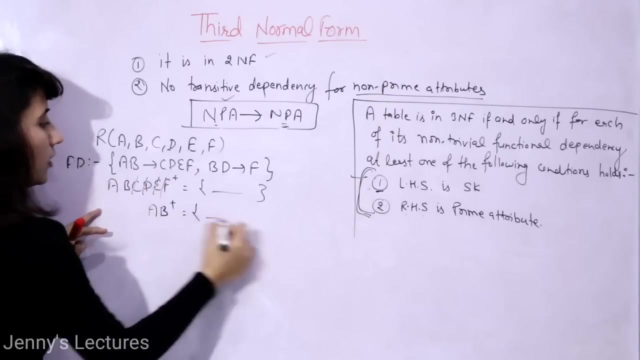 so we have a, b. so using a b i can determine c, d, e, f. so i can discard from here. right, can I discard anything else? b, d is determining f, but we don't have, we have only b, we don't have d, right, so obviously we can, cannot discard now anything. so now a, b. you can find out a b closer. 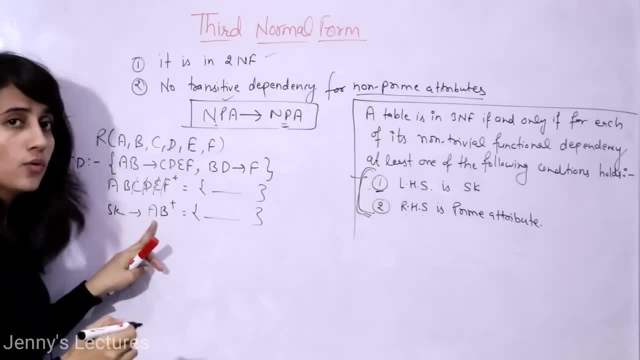 would also contain all the attributes. so this is worth a super key. now find out it is a candidate key or not. how to find out a- b closer. now lets say how to find out a- b closer. how to find out a- b closer. proper subset would be a and b. check out these are super key or not? a closer and b closer. a closer. 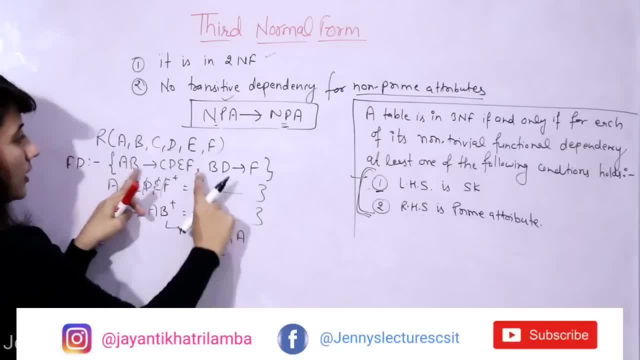 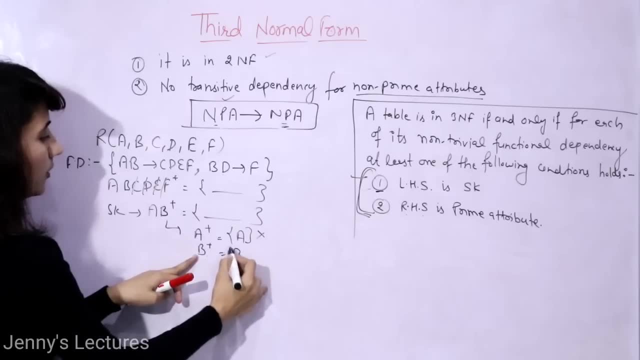 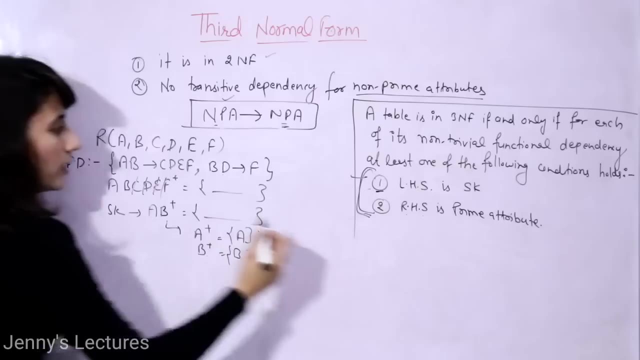 will determine itself a, nothing else, because here both a, b is determining c, d, e, f. but we have only a, not b, right? so this is not a super key. now b, closer, will determine b, only b, so this is also not a super key. so you can say that a, b is candidate key. right now we go to one candidate. 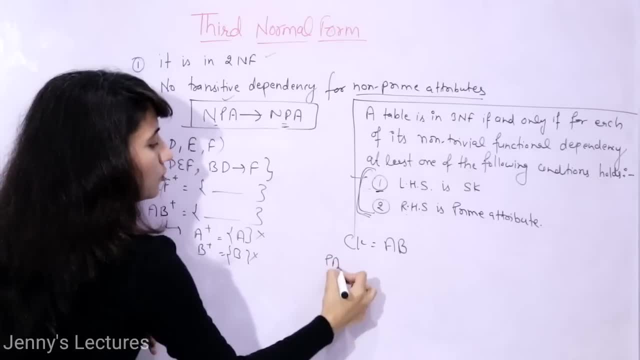 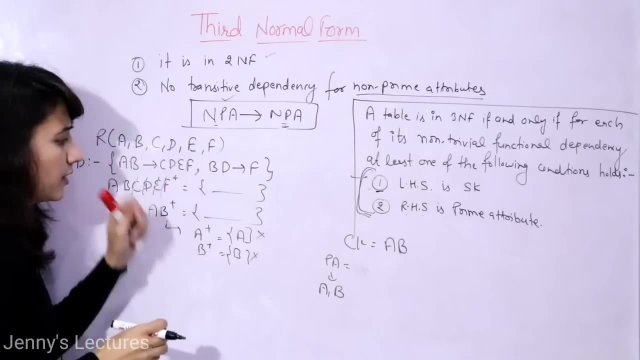 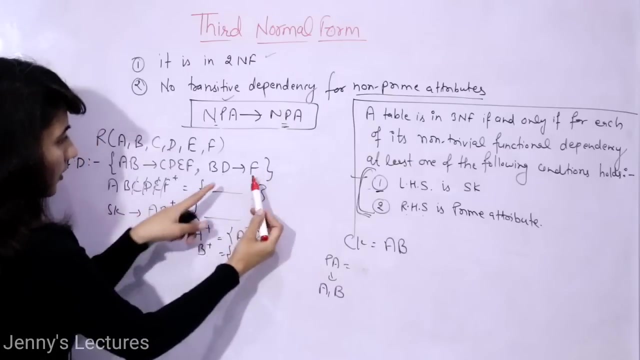 key that is a, b and prime attributes are here: a comma, b. now check more candidate keys. are there or not? how to check prime attributes: check out the prime attributes: are available on the right hand side or not. is a available on the right hand side? no. is b available on the right hand side? no. 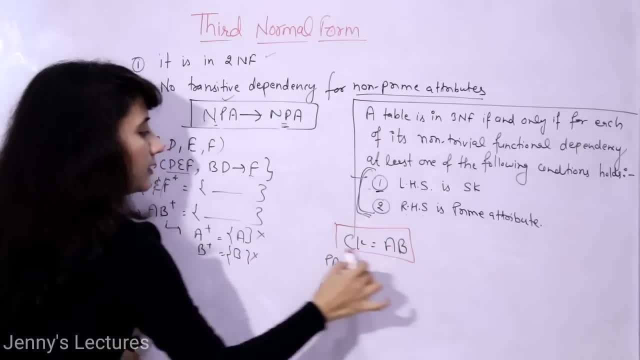 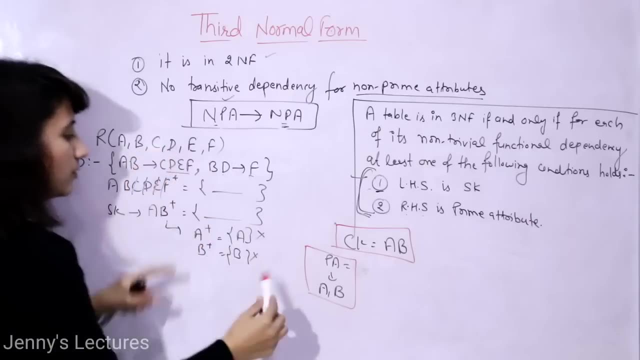 it means there is only one candidate key. no more candidate keys are present in this relation. right and prime attributes are a and b. non-prime attributes are available on the right hand side. no, it means there is only one candidate key. no attributes are C, D, E, F. right now, check out for this dependency. is this type of? 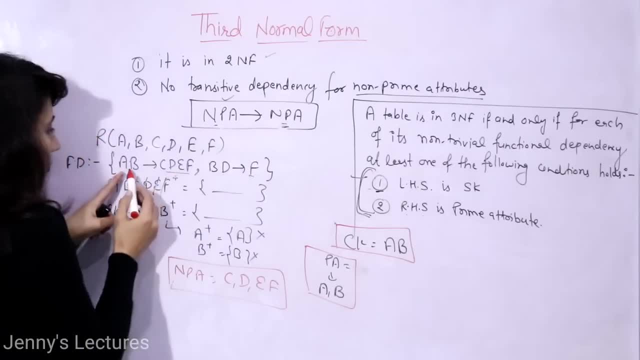 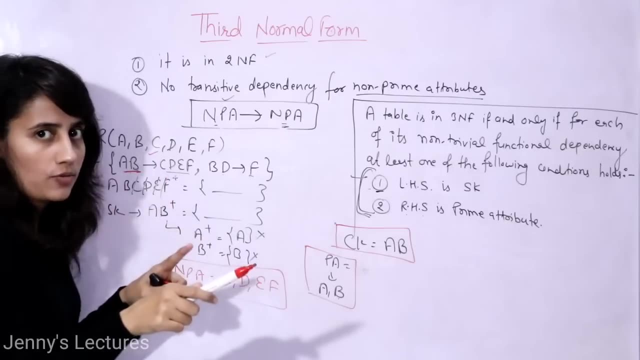 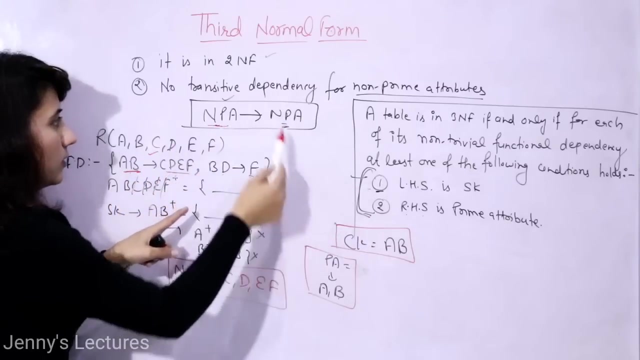 type of dependency present here or not see. first of all, this thing is this: AB is non prime attribute. no, AB are prime attribute. so this is what? not a transitive dependency right? no need to check the right hand side, because if this side is not NPA, so no need to check for this side. now check for this. 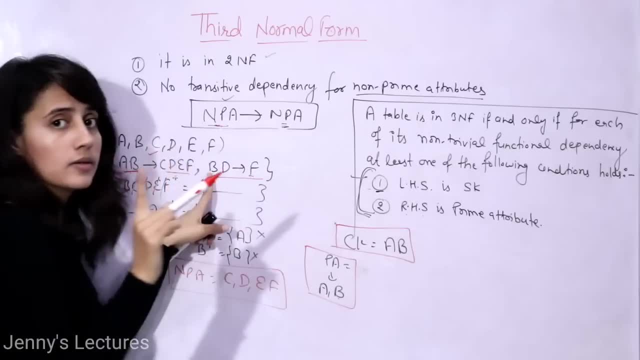 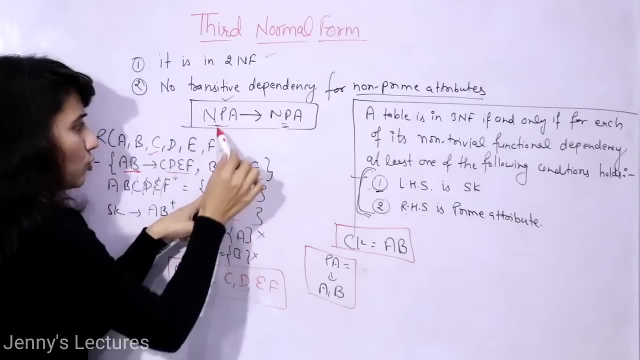 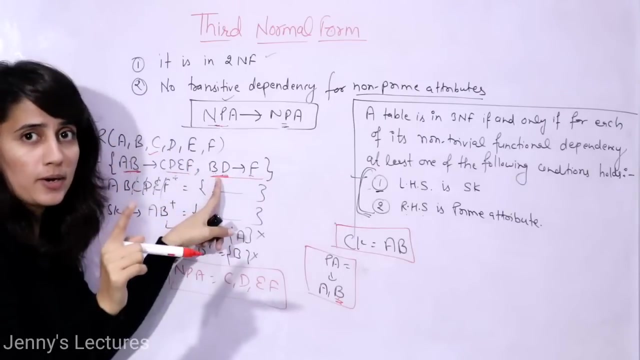 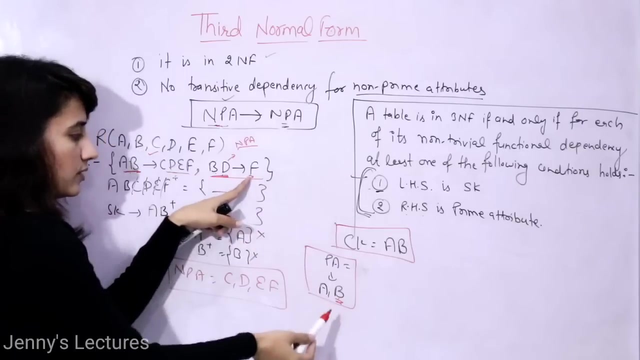 dependency: see B and D. now here, see this point. you need to clear out this point very carefully. both B and D, is this non prime attribute? now we will say that B is prime attribute, right, but D is not a prime attribute. so this will consider as non prime attribute. and right hand side is F. F is what it's: a non prime. 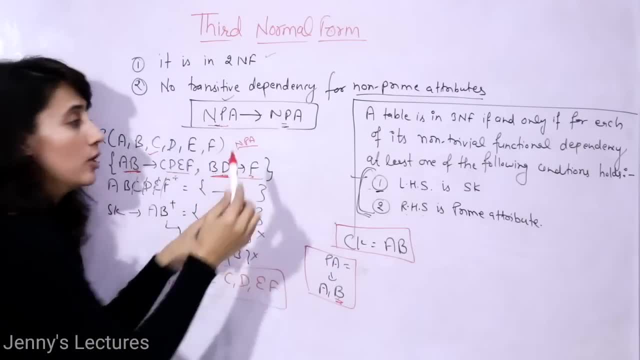 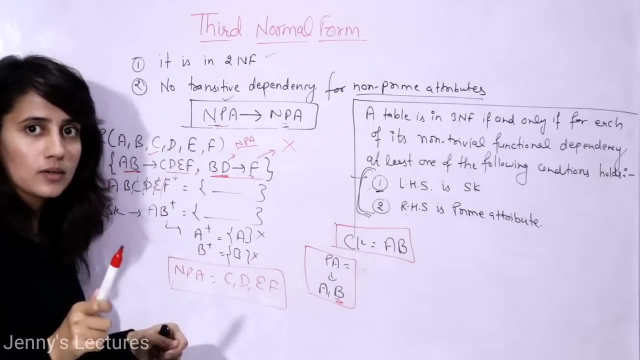 attribute. so here also non prime attribute, here also non prime attribute. so this is violating the condition. so this relation is not in third normal form, right, I hope you got now. if you you'll find the mix of prime and non prime attribute, then you will consider it what a non prime attribute complete. 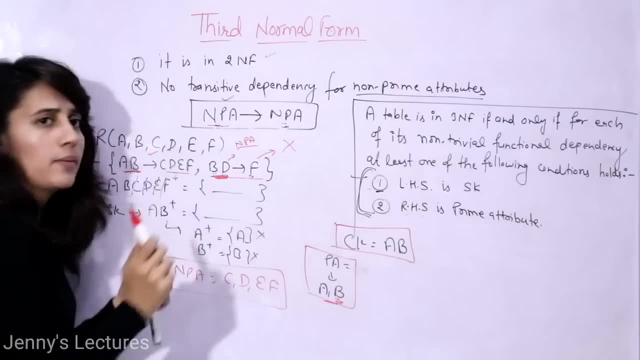 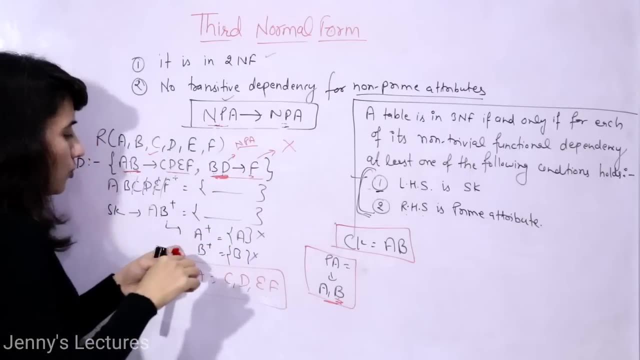 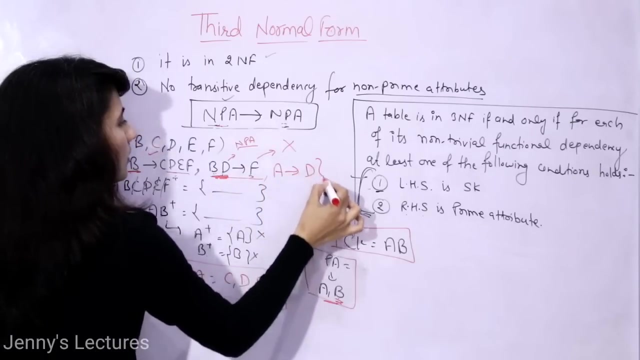 because B, D, complete, is not prime attribute. D is not in prime attribute, so we'll consider it as non prime attribute, right? so this is not in third normal form. suppose I am going to modify it a little bit. suppose I have. I am having a warm functional dependency, that is, A determine D. so now check for this one. 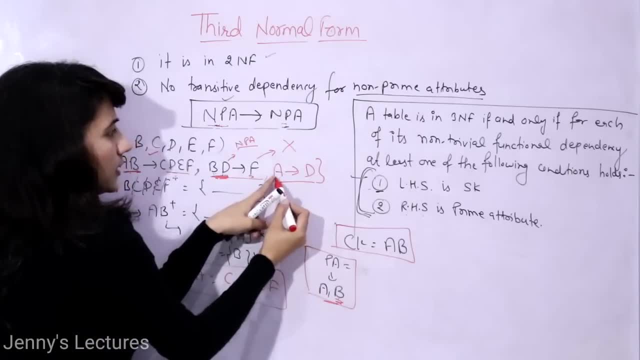 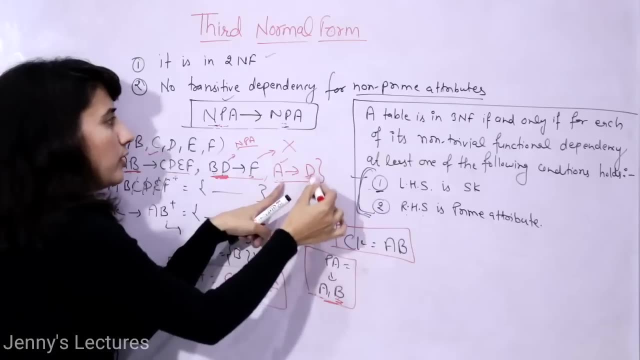 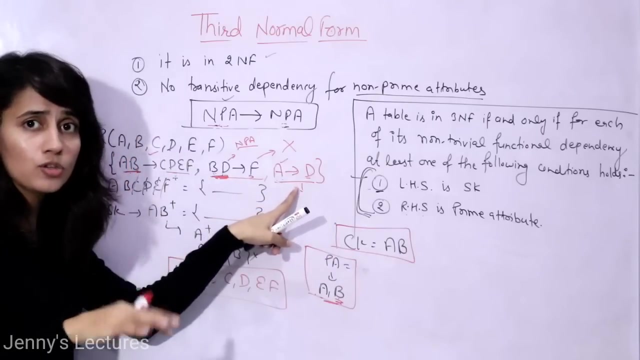 also suppose I am taking this one also. so for this functional dependency, left hand side is non prime attribute. no, it is what prime attribute A is what prime attribute right. so no need to check the right hand side. this is not violating that property. this is what we can. we cannot say that this is a transitive. 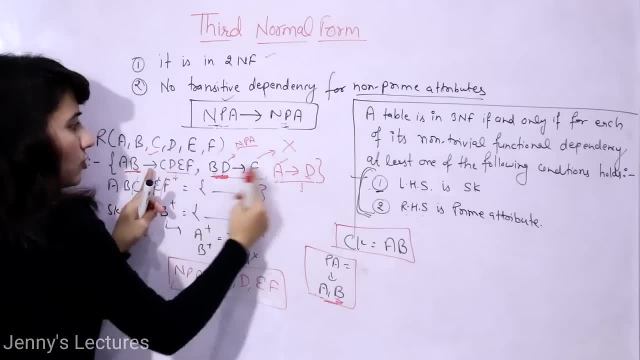 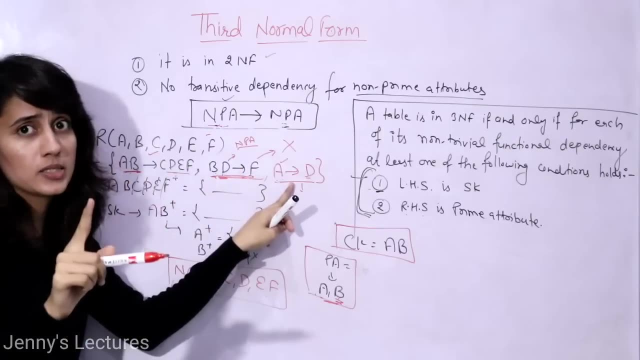 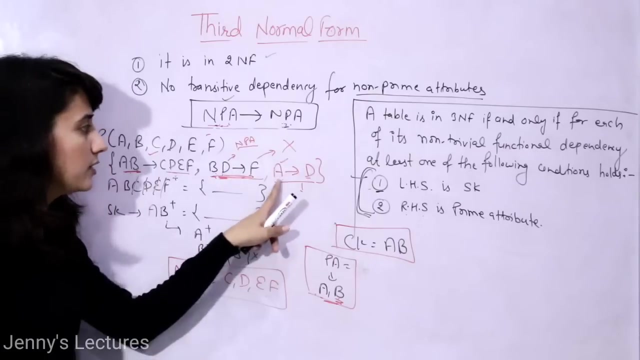 dependency right here. only, which dependency is violating the condition? because of this dependency, this relation is not in third normal form B, not because of this dependency right. make this thing very clear: that both side should be non prime attribute, non prime attribute and this A is prime attribute. so no need to check this one or you can check this one left. 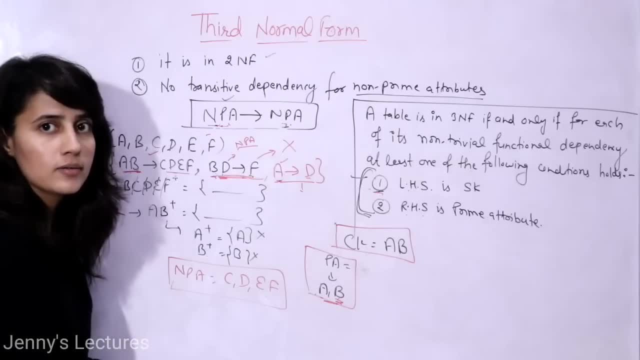 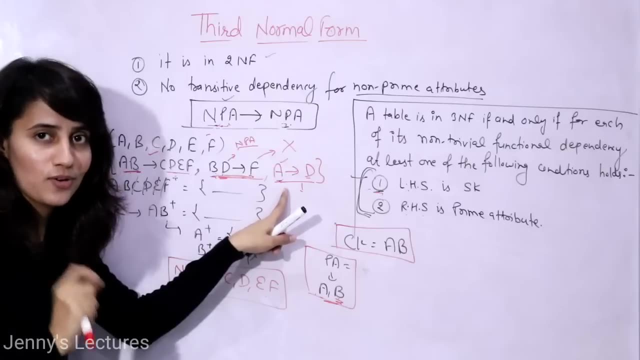 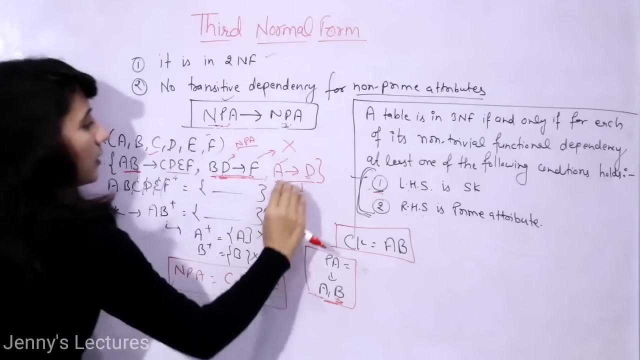 hand side is super key. yes, A is super key, so no need to check the right hand side, right. so now see if this is a case. if this is a case, then check for the second normal form here, because this relation is now in, not in second normal form, right see, A is determining D, A is what. 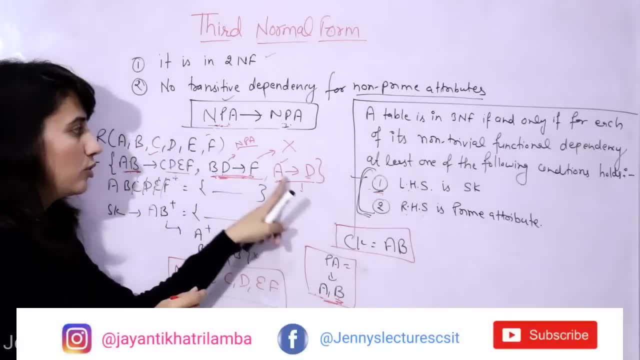 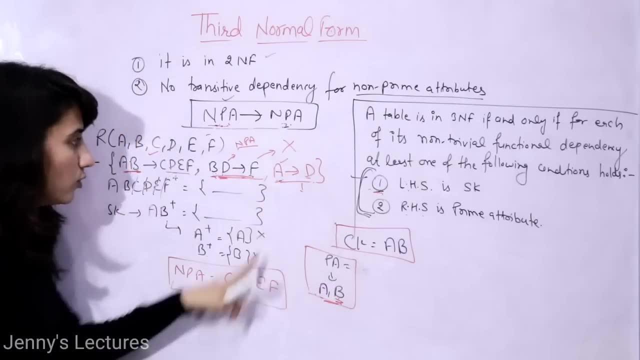 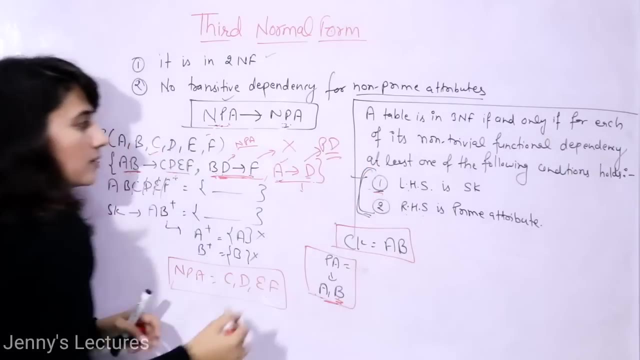 candidate key is AB, or you can say primary key is also AB and a proper subset of candidate key is A and this is determining a non prime attribute. D is what a non prime attribute. so this is a case of partial dependency. here this is partial dependency. so if this is a 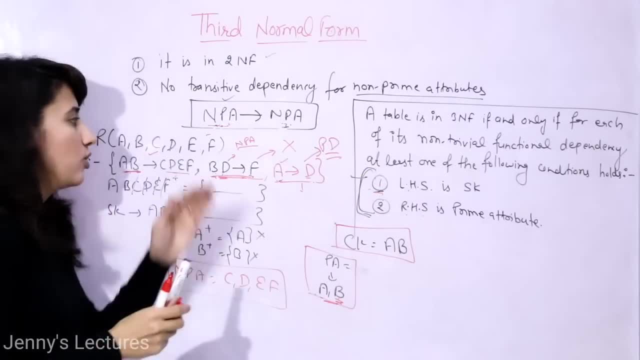 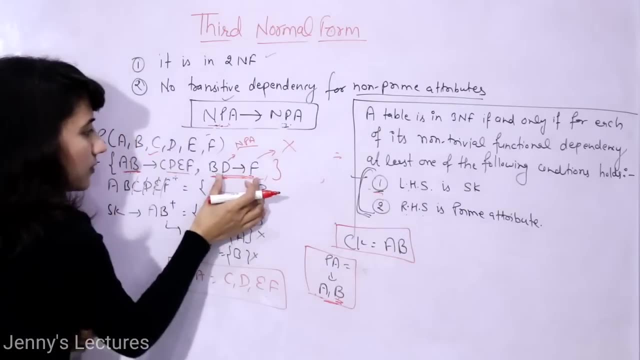 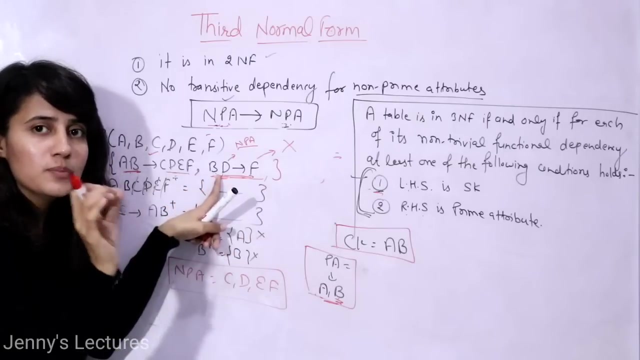 case, then this relation is not in second normal form, So definitely it cannot be in third normal form Right Now here. obviously I am not taking this one Now. check This is partial dependency or not. C, BD- Is it a proper subset of candidate key? Candidate key is AB. 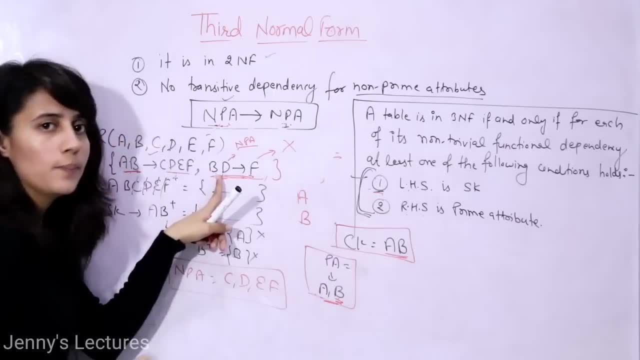 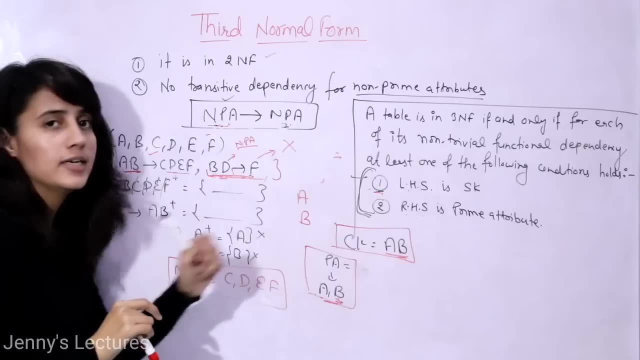 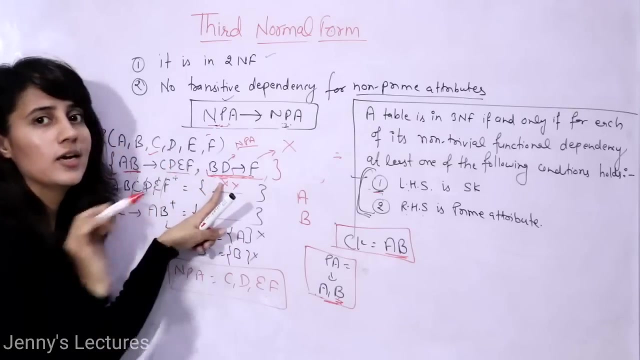 Proper subset of candidate key. One is A, One is B, Although we have B here But we have D also. This complete should be a proper subset of candidate key. So this is not a proper subset of candidate key Right. So this is not a partial dependency Right. So this is in second normal form. 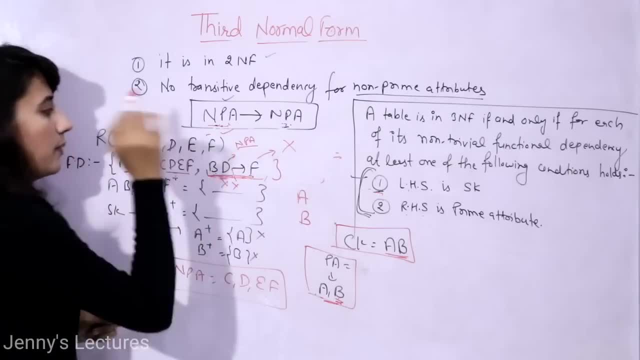 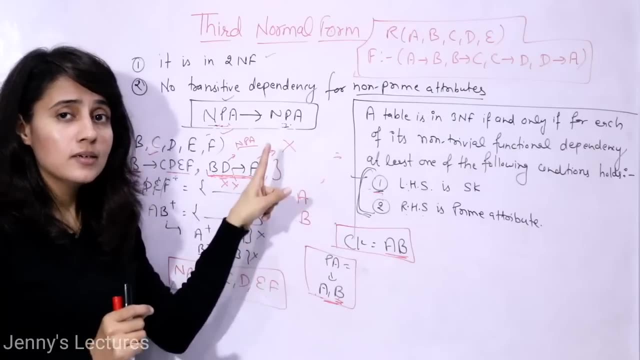 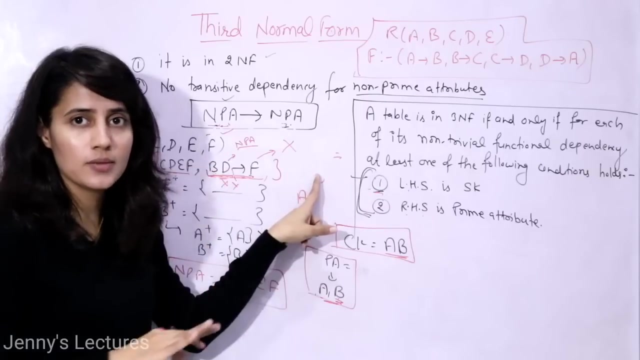 But not in third normal form, Because this is transitive dependency. I hope now you got all the points about this. So now how you can say that third NF is better than second NF. In two NF we have one anomaly, that is update anomaly, Because of some redundancy there. 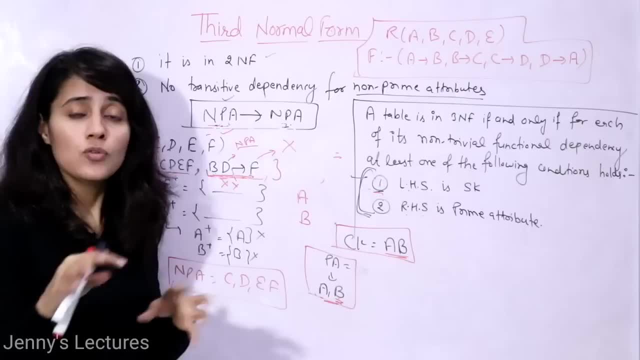 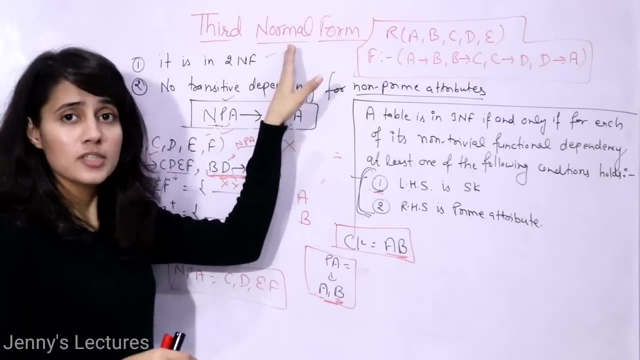 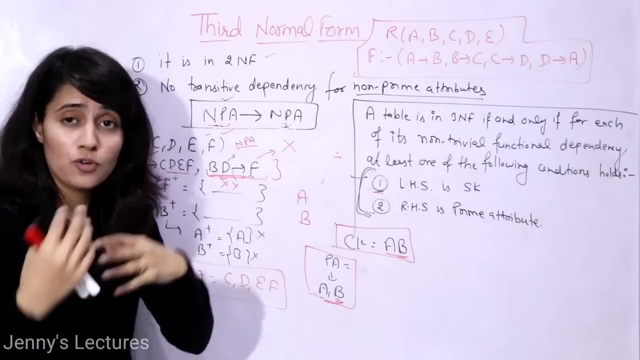 Right, That is drawback. So now third NF will remove all the anomalies: Insert, Delete, As well as update anomaly. So now you can say that That is why we say that This third normal form is adequate normal form for your database, Means if your database is in third NF. 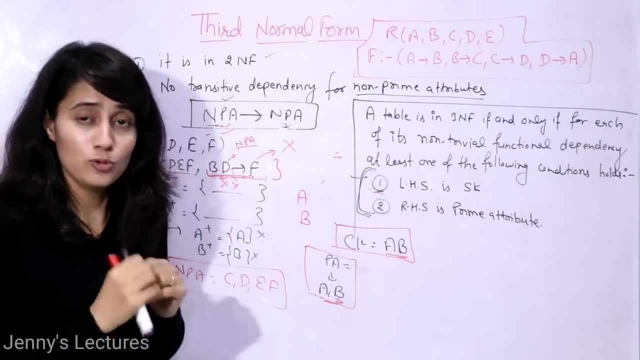 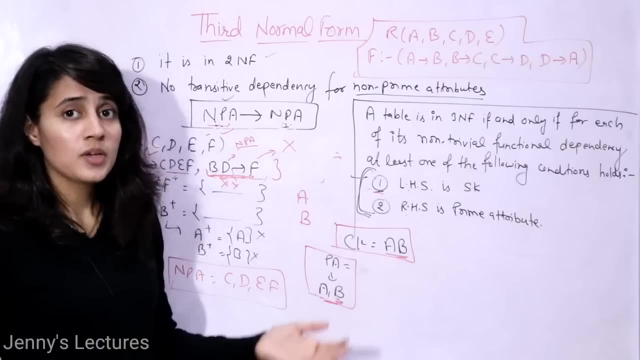 Then you can say that it is a good database design. Although we have more normal forms, are there BCNF, Fourth, Fifth, DKNF? That also we will discuss one by one later. Now I hope you got What is third normal form And how to find out that particular relation is in third NF or not. 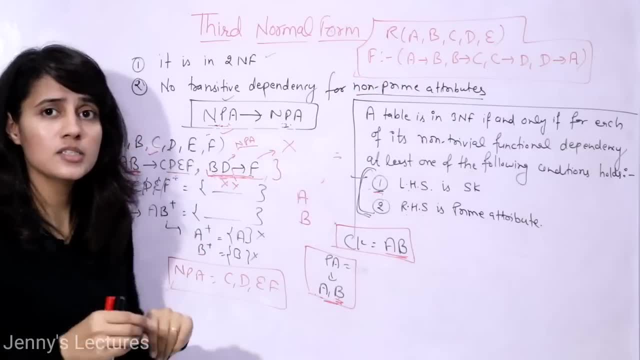 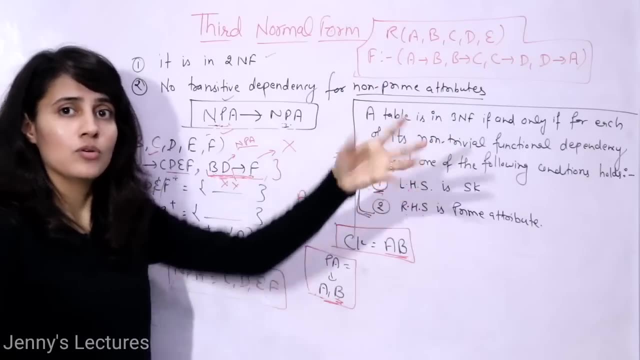 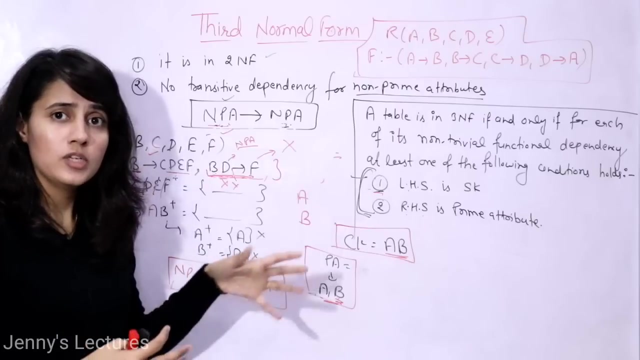 Now, this is question for you. This is the relation. These are functional dependencies And you need to check out: is this relation Is in second normal form as well as in third normal form, or not? Right, You need to tell me. Fine, Now, if you want me to discuss more questions on these normal form. 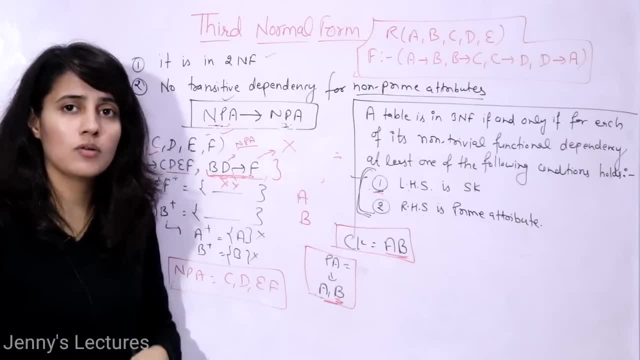 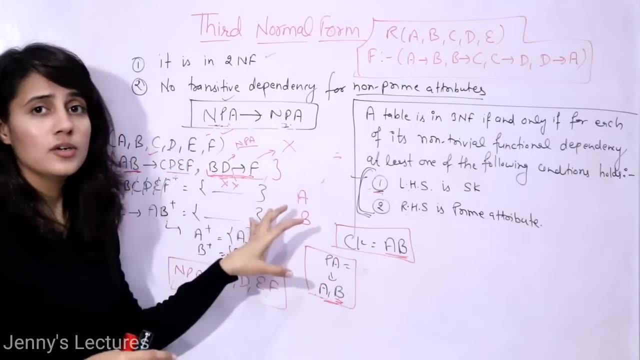 You can mail me your questions on my mail id Or you can just tell me in the comment box. I will discuss some more questions on these normal form. So now, how to convert a given relation in Into third NF, Third normal form, That thing we will discuss later, after discussing the decomposition process. 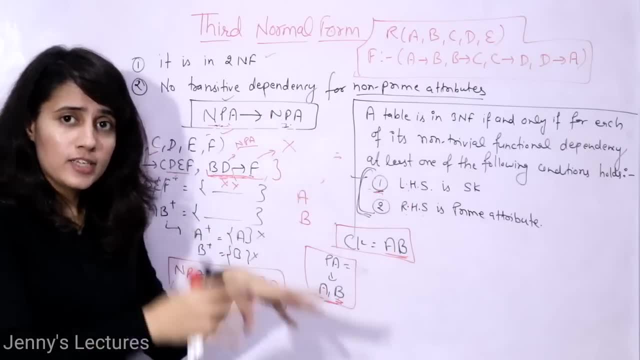 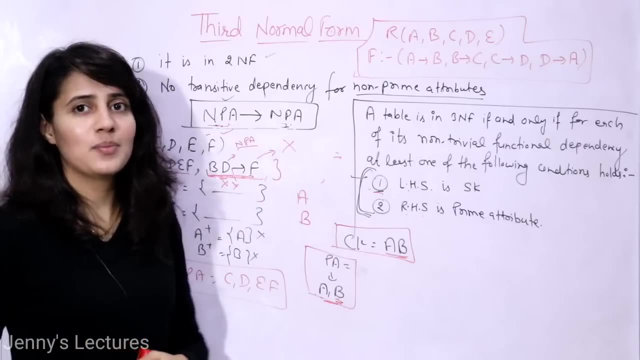 Means lossless and docile decomposition. Right In the next video I will discuss What is BCNF, And after that I will discuss about decomposition process. So now I will see you in the next video. Till then, bye, bye, take care.